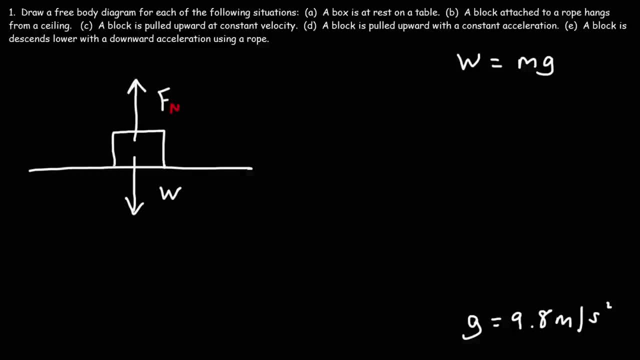 The normal force is always perpendicular to the surface. It's at a 90 degree angle. Now, because these two are equal, because the box is at rest, the normal force is going to be equal to mg. Now, because they're equal, you want the length of these two arrows to be approximately the same. 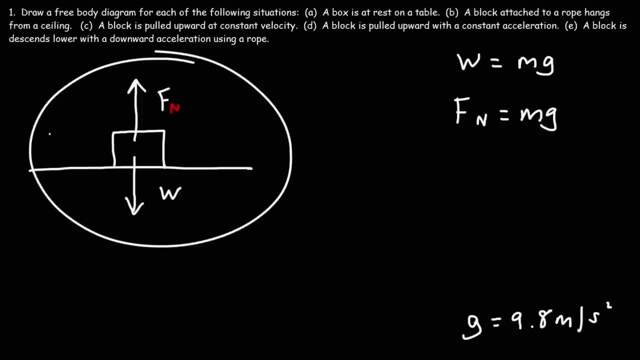 So that's it for part a. This is the free body diagram that we can draw to represent the box resting on a table. Okay, so now let's move on to part b. A block attached to a rope hangs from a ceiling. Draw the free body diagram for that. 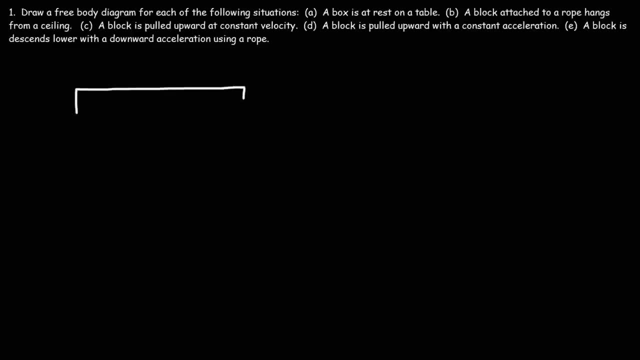 So let's say, this is the ceiling and we're going to have a block that is attached to one rope that connects the block to the ceiling. So what forces are acting on this block? So we have the weight force, which we can call W or you can say F, gravity, and we also have an upward 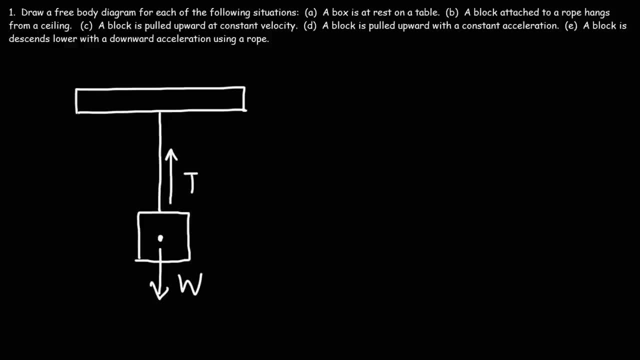 and downward tension force. Now this block is at rest. It's not accelerating upward or downward, so the net force in the y direction is 0. Therefore these two arrows should be of the same length. So in this example the tension is equal to the weight force and the weight force is mg. 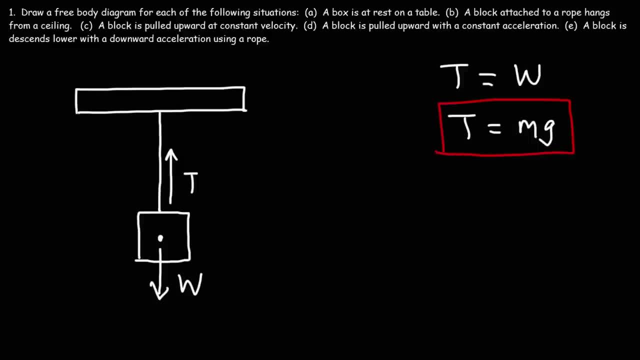 So the tension in the rope is simply mg. Tension is always the force, V chord that acts through a rope. Now what about part C? A block is pulled upward at constant velocity. To pull a block upward we need a rope. So the block is moving upward at constant velocity. We're gonna have a. 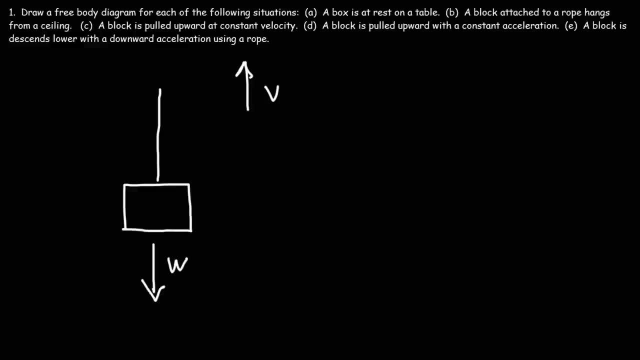 weight force and we're gonna have an upward tension force. Are these two forces the same or are they different? At constant velocity, what is the acceleration? The acceleration is zero at constant velocity. The net force in the y-direction is going to be the difference between a tension and the 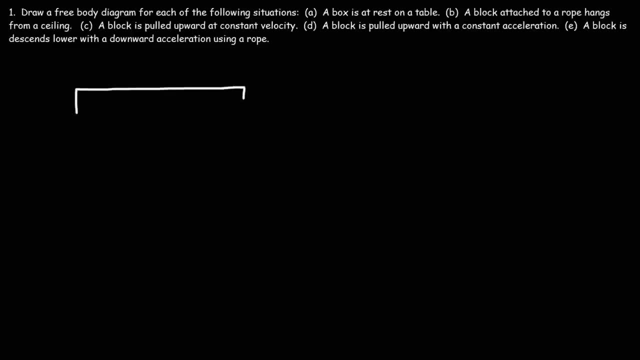 So let's say, this is the ceiling and we're going to have a block that is attached to one rope that connects the block to the ceiling. So what forces are acting on this block? So we have the weight force, which we can call W or you can say F, gravity, and we also have an upward 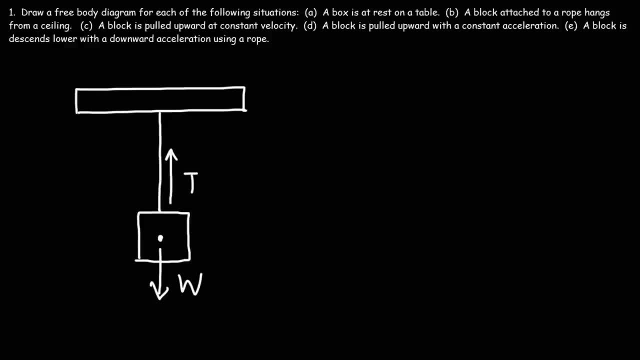 force, which is the tension force. Now this block is at rest, It's not accelerating upward or downward, So the net force in the y direction is zero. Therefore these two arrows should be of the same length. So in this example the tension is equal to the weight force and the weight force. 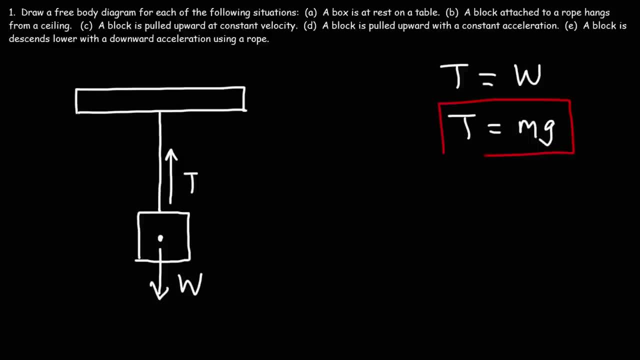 is mg. So the tension in the rope is simply mg. Now what about part c? A block is pulled upward at constant velocity. To pull a block upward we need a rope. So the block is moving upward at constant velocity. We're going to have a weight force and we're going to have an upward tension force. 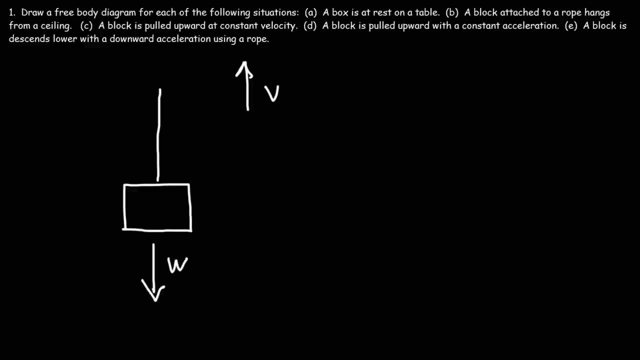 Are these two forces equal to the force that is acting on the ceiling? Are they the same or are they different? At constant velocity, what is the acceleration? The acceleration is zero at constant velocity. The net force in the y direction is going to be the difference between the tension and the weight. 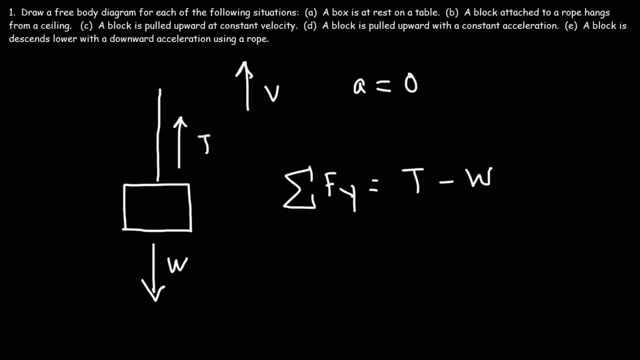 force And according to Newton's second law, the net force, which is the sum of the forces, it's going to equal to m times 8.. So we can replace this with ma. Now, if the acceleration is zero, the net force is going to be zero. 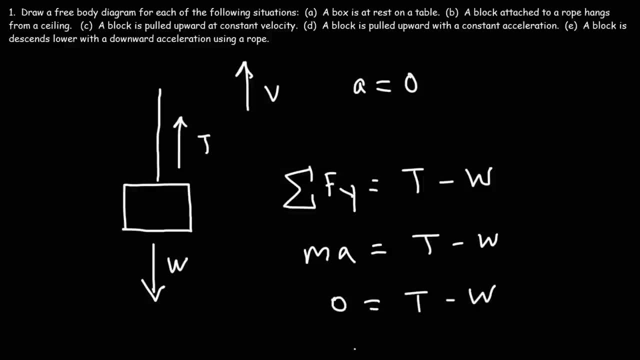 Adding w to both sides, we can see that the weight force and the tension force they're the same. So by constant velocity these two forces will cancel out because the acceleration is zero. So therefore the length of the two arrows should be the same. So that's the tension force and the force that is acting on the ceiling. 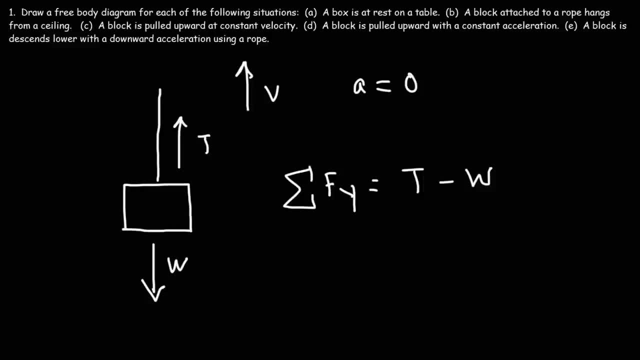 weight force And according to Newton's second law, the net force, which is the sum of the forces, it's going to equal to m times 8.. So we can replace this with ma. So we can replace this with ma. Now, if the acceleration is zero, the net force is going to be zero. Add in W to 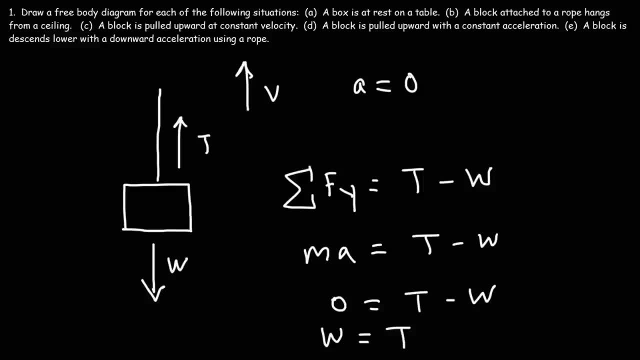 both sides. we can see that the weight force and the tension force they're the same. So by constant velocity these two forces will cancel out because the acceleration is zero. So therefore the length of the two arrows should be the same. So that's, the tension in this problem is equal to the weight force, which is equal. 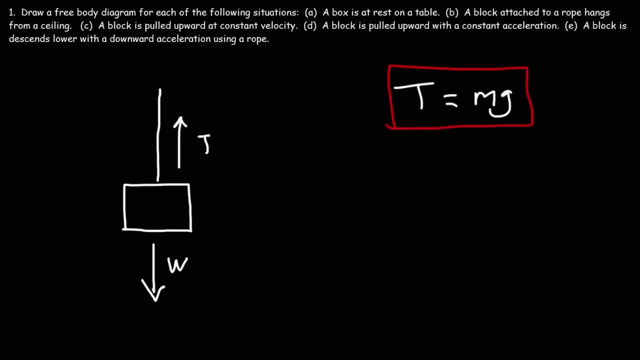 to mg. So that's all we need to do to show the free body diagram for part C. Now let's move on to part D. This time a block is pulled upward with a constant acceleration, So the equation changes. So we can still write this equation. 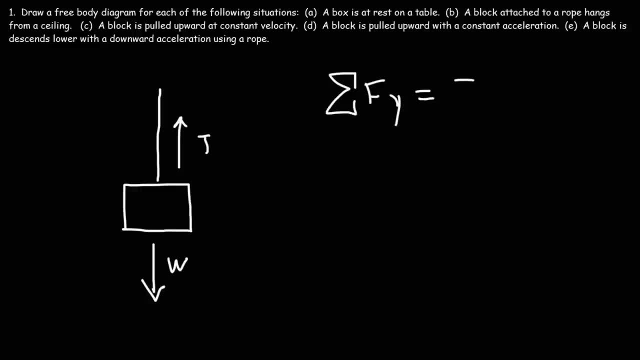 The sum of the forces in the y-direction. that's still going to be equal to tension minus the weight force, And the net force in the y-direction is going to be ma. You can put a sub y if you want to for acceleration in the y-direction, So this: 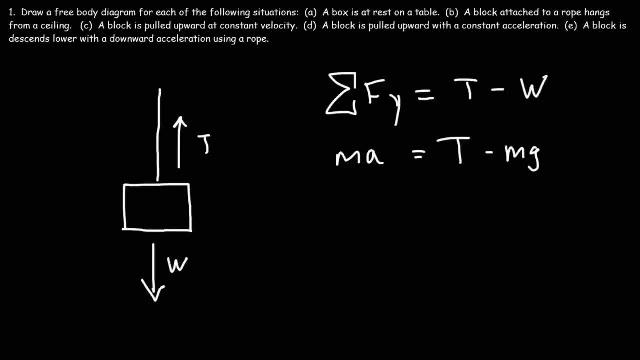 is tension minus mg. If we move mg to the other side, notice that we have ma plus mg. So that's how you can calculate the tension for this example. if there's a upward acceleration, So notice that tension is greater than mg. It's mg plus. 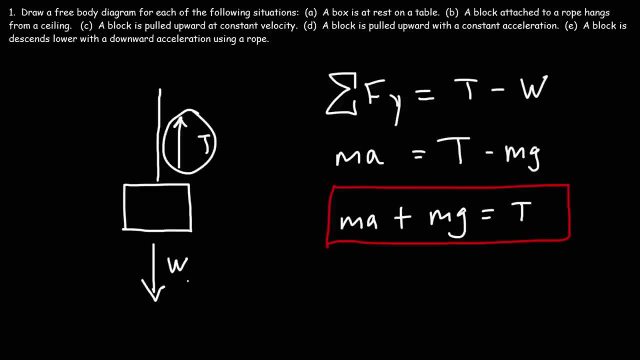 ma. Therefore this arrow has to be longer than the arrow for the weight force or F gravity. So let's make this arrow significantly bigger than the other one. So if t is bigger than w, there's going to be an upward net force that's going to 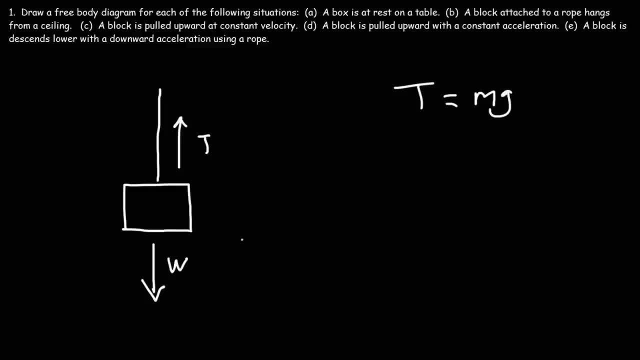 in this problem is equal to the weight force, which is equal to mg. So that's all we need to do to show the free body diagram for part C. Now let's move on to part D. This time a block is pulled upward with a. 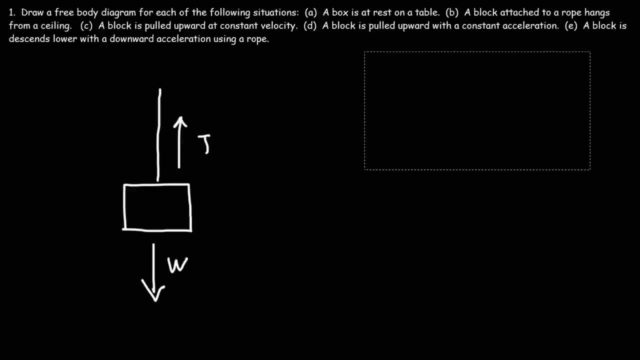 constant acceleration. So the equation changes. So we can still write this equation: The sum of the forces in the y direction that's still going to be equal to tension minus the weight force, And the net force in the y direction is going to be ma. You can put a sub y if you want to. 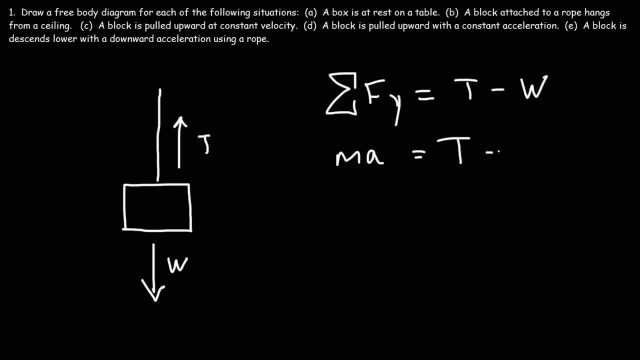 for acceleration in the y direction. So this is tension minus mg. If we move mg to the other side, notice that we have ma plus mg. So that's how you can calculate the tension for this example if there's an upward acceleration. So notice. 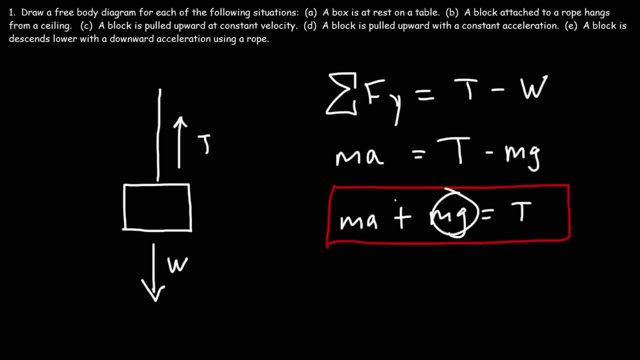 that tension is greater than mg, It's mg plus ma. Therefore this arrow has to be longer than the arrow for the weight force or F gravity. So let's make this arrow significantly bigger than the other one. So if T is bigger than W, there's going to be an upward. 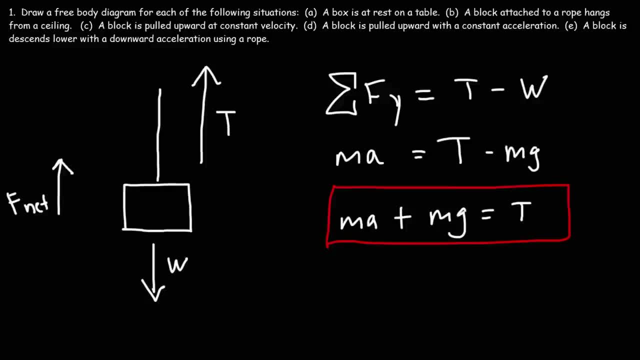 net force That's going to accelerate the block upward. Now what about E A block? let's take this word out. A block descends lower with a downward acceleration using a rope. So in this case, the acceleration is negative if it's going down. 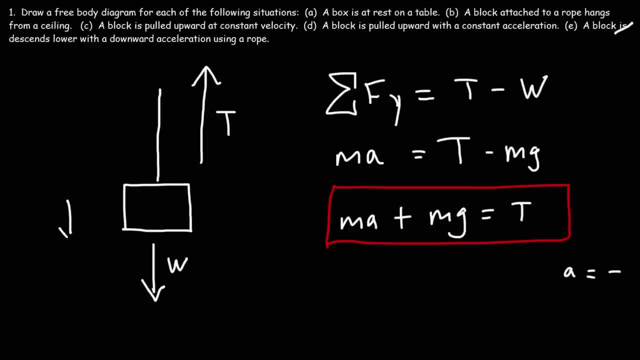 The net force is going to be in the downward direction, Because it's descending lower with a downward acceleration, And the only way that's going to happen is if W is greater than T. So we're going to make this arrow smaller And we're going to make this one bigger. 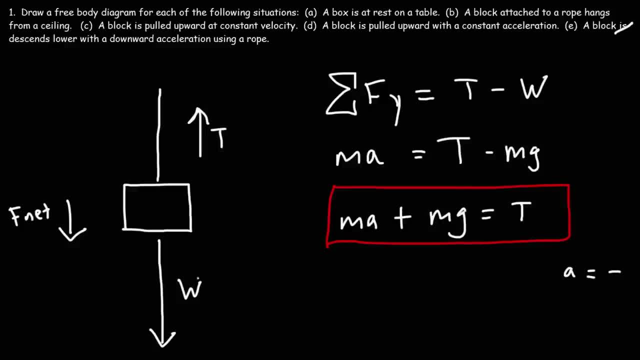 So now we have a downward acceleration because the weight force or the force of gravity is smaller. The vector could get those 2 Jazzed things bigger. So you can different. the die華 brosca diabetes does something wrong, so we're going. taltiva Z. 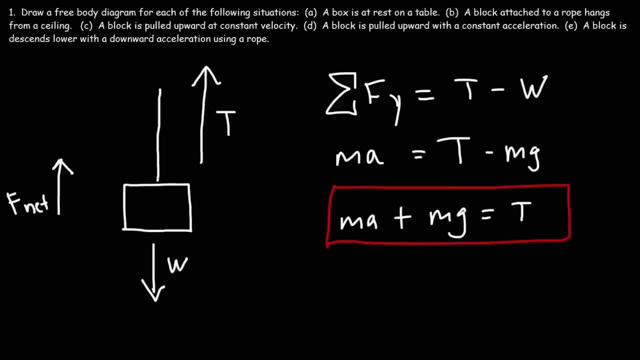 accelerate the block upward. Now what about E, A block? let's take this word out. a block descends lower with a downward acceleration using a rope. So in this case, the acceleration is negative. if it's going down, The net force is. 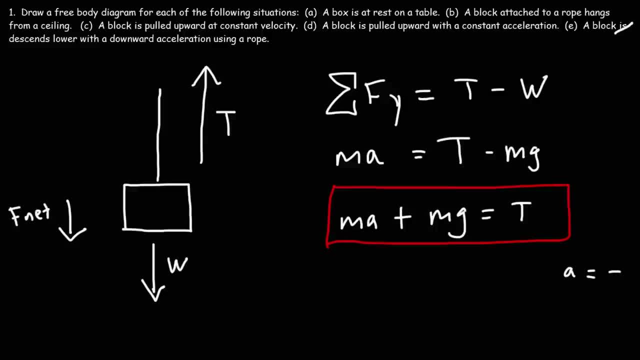 going to be in the downward direction, Because it's descending lower with a downward acceleration, And the only way that's going to happen is if w is greater than t. So we're going to make this arrow smaller, We're going to make this one bigger. So now we have a. 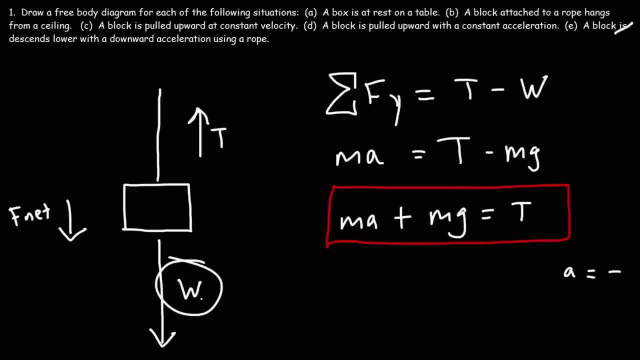 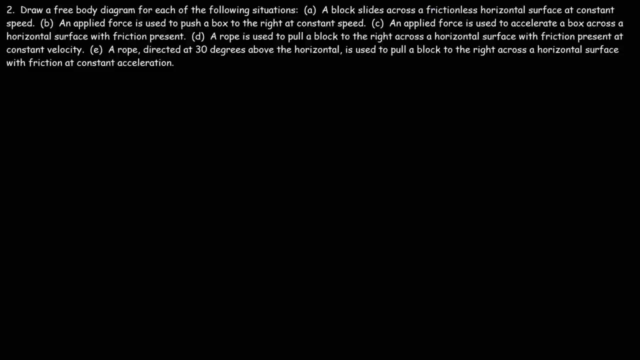 downward acceleration because the weight force or the force of gravity is greater than the tension force. So that's it for E. That's the free body diagram that correlates to that situation. So now let's work on some more examples For part A. we have a block that slides across a frictionless horizontal surface at 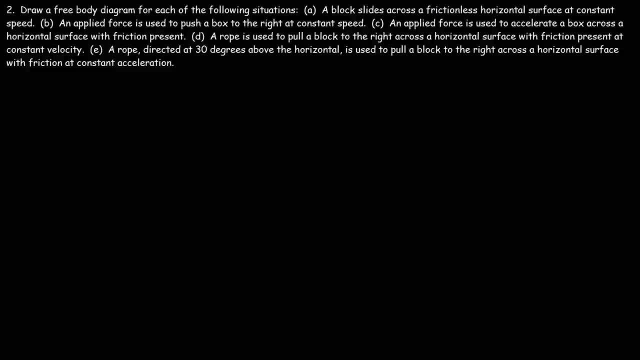 constant speed. Go ahead and draw a free body diagram for that situation. So first we have a horizontal surface and then we have a block on that surface, And let's say it's moving to the right at constant speed. What forces are acting on this block? Well, anytime you have an object resting on a surface, 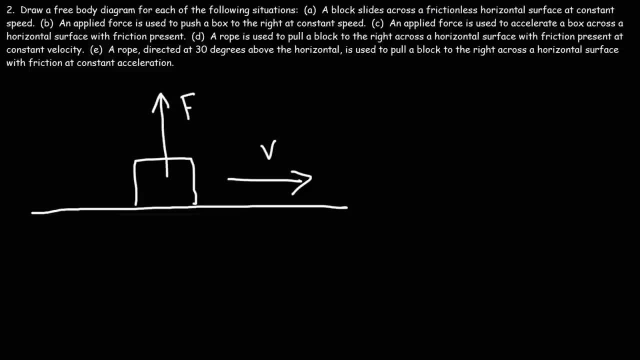 there's going to be an upward normal force And that upward normal force is going to be equal to the weight force. So we need to make sure the lengths of those two arrows are the same. Are there any forces in the x-direction If the object is moving at constant velocity? 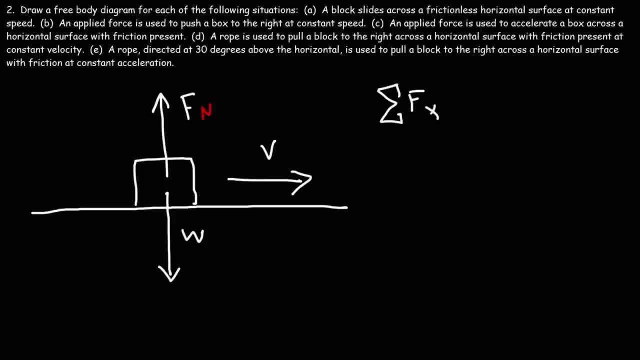 the net force, or the sum of the forces in the x-direction will be zero. There's no friction slowing this down, So we don't have friction. Therefore there's no applied force accelerating it to the right, So there's no forces in the x-direction here. So this is all we could. 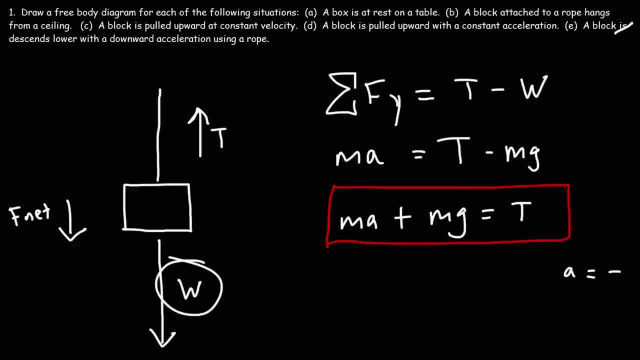 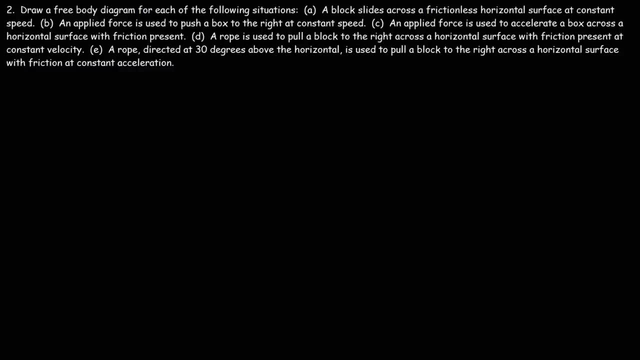 perfectcı is greater than the tension force. So that's it for E. That's the free body diagram that correlates to that situation. So now let's work on some more examples For part A. we have a block that slides across a frictionless horizontal surface at constant speed. Go ahead and draw a free body. 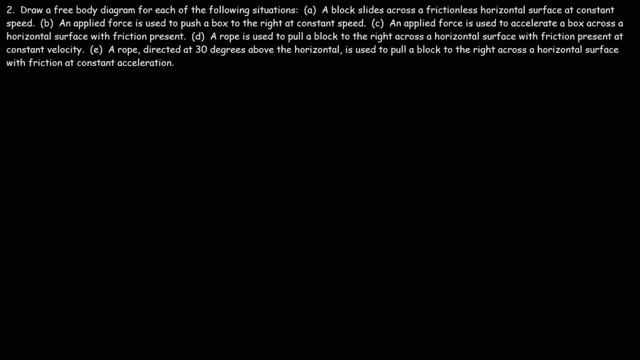 diagram for that situation. So first we have a horizontal surface and then we have a block on that surface and let's say it's moving to the right at constant speed. What forces are acting on this block? Well, anytime you have an object resting on a surface, there's going to be. 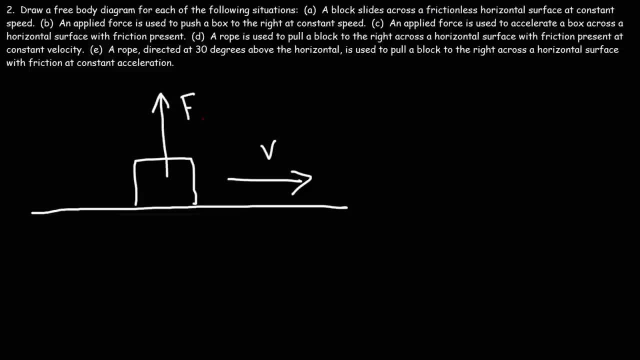 an upward normal force, and that upward normal force is going to be equal to the wave force. So we need to make sure the lengths of those two arrows are the same. Now, are there any forces that are acting on this block? Well, if you have an object resting on a 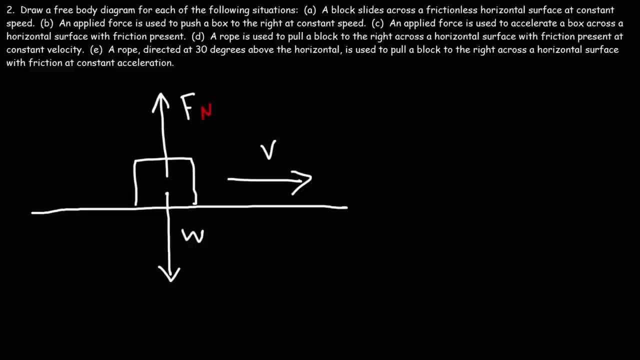 surface, there's going to be any forces in the x direction. If the object is moving at constant velocity, the net force, or the sum of the forces in the x direction, will be zero. There's no friction slowing this down, so we don't have friction. Therefore there's no applied force accelerating. 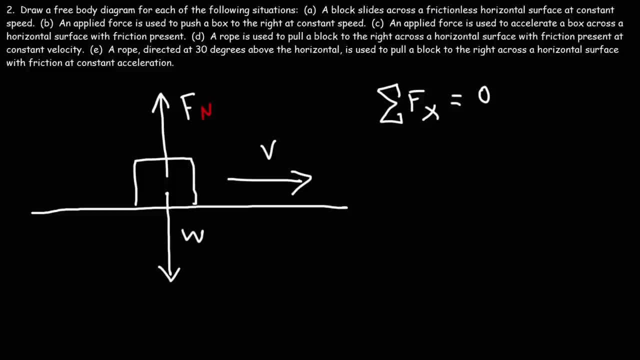 it to the right. So there's no forces in the x direction here. So this is all we could show for the free body diagram for part A. Now let's move on to part B. So in part B we have an applied force that is used to push the box to the right at constant speed. 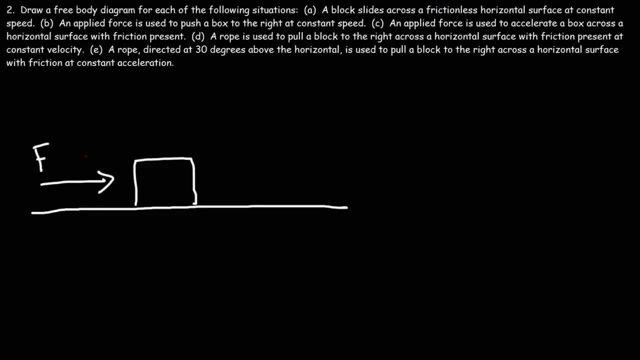 So this is going to be the applied force. Now we still have a normal force, So that's going to be the applied force. So the applied force is going to be present And the wave force is still there. Now the box is moving at constant speed. If it's moving at constant speed, the acceleration is zero. 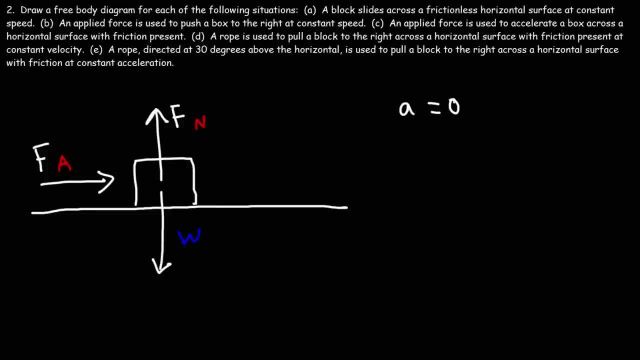 So the forces in the x direction must be balanced, because the net force is zero in the x direction. So therefore, if the net force in the x direction must be zero, what other forces do we have? The only other force that could be acting in the x direction must be friction. 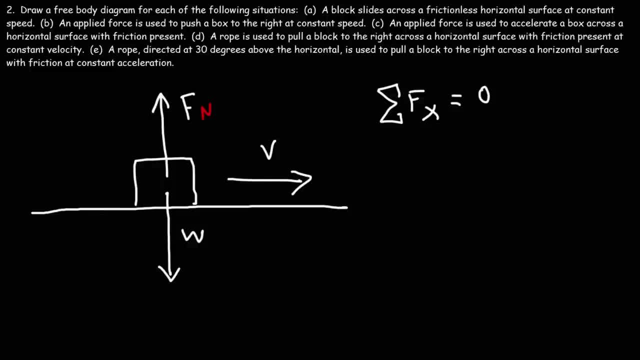 show for the free body diagram for part A. Now let's move on to part B. So in part B we have an applied force that is used to push the box to the right at constant speed. So this is going to be the applied force. Now we still have a normal force. So 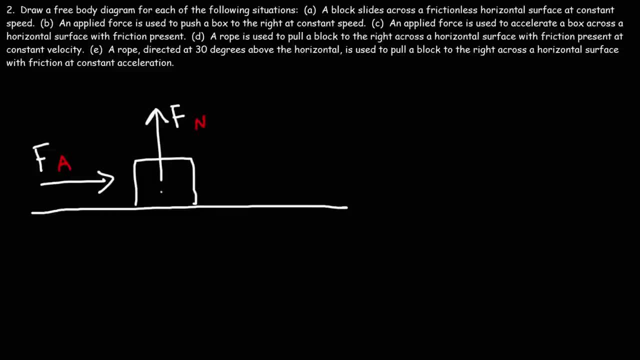 that's going to be present And the weight force is still there. Now the box is moving at constant speed. If it's moving at constant speed, the acceleration is zero. So the forces in the x-direction must be balanced, because the net force is. 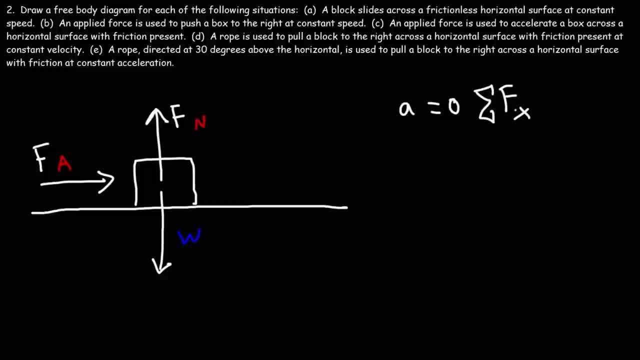 zero in the x-direction. So therefore, if the net force in the x-direction must be zero, what other forces do we have? The only other force that could be acting in the x-direction must be friction. 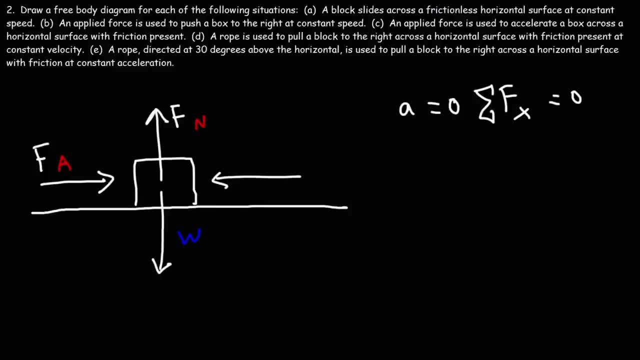 Now there's two types of frictional forces. There's static friction and kinetic friction. The word kinetic indicates that the object is in motion, And since this object is moving at constant speed, kinetic friction is active, which we'll call FK. 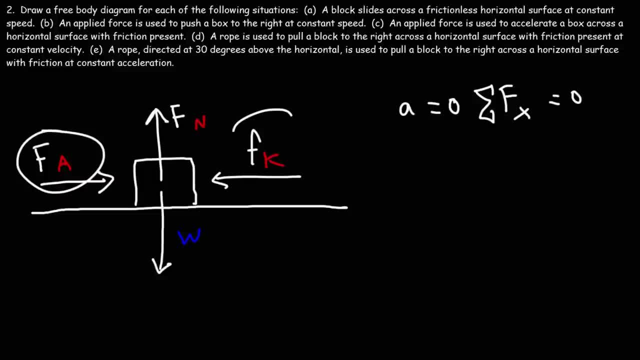 Now these two forces must be equal in order for the acceleration to be zero. So the arrow, these two arrows, have to have the same length. So that's the answer for Part B. Part C: An applied force is used to accelerate a box across a horizontal surface with friction present. 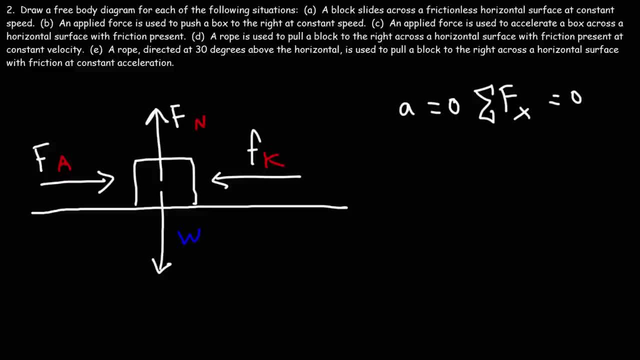 So friction was already present in the x-direction. But this time the box is not moving at constant speed, It's accelerating. So the acceleration is not zero. Because we have an acceleration, there's going to be a net force to the right. 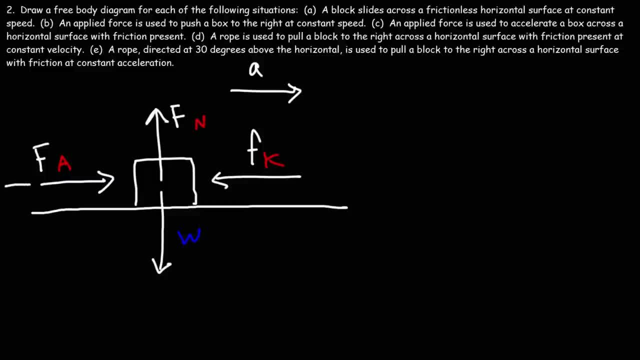 And the only way that's going to happen is if the applied force is greater than FK. So kinetic friction Has to be relatively small compared to the applied force so that we can have a net acceleration to the right. So this is going to be the free body diagram for Part C. 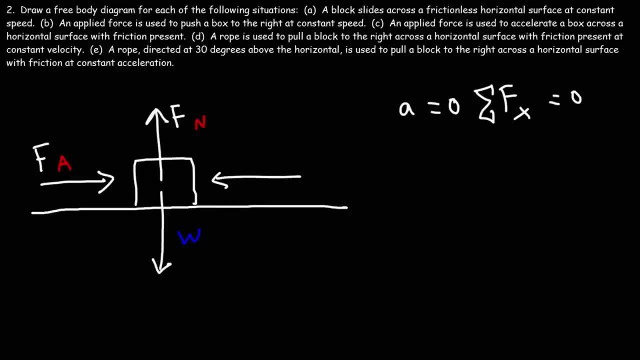 Now there's two types of frictional forces. There's static friction and kinetic friction. The word kinetic indicates that the object is in motion, And since this object is moving at constant speed, kinetic friction is active, which we'll call FK. Now these two forces must be equal in order for the acceleration to be zero. 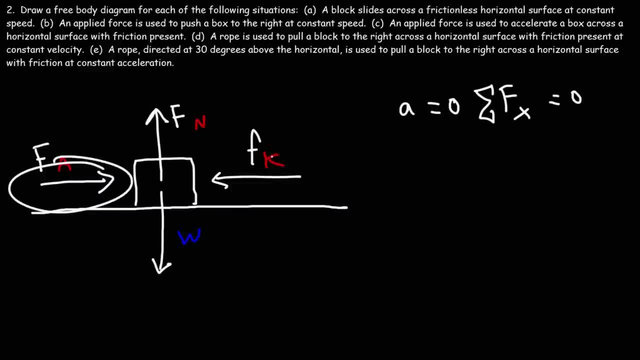 So the arrow, these two arrows, have to have the same length. So that's the answer for Part B. Part C, an applied force is used to accelerate a box across a horizontal surface with friction present. So friction was already present in Part B. 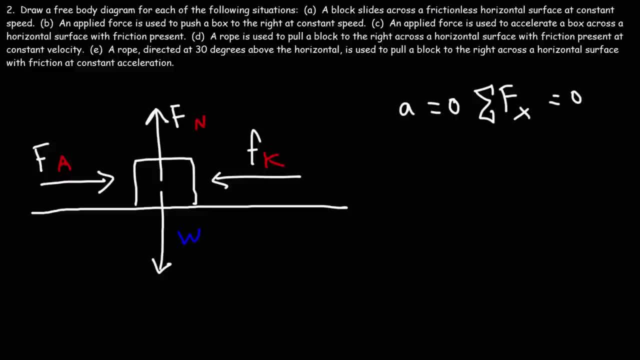 But this time the box is not moving at constant speed, it's accelerating. So the acceleration is not zero. Because we have an acceleration, there's going to be a net force to the right, And the only way that's going to happen is if the applied force is greater than Fk. 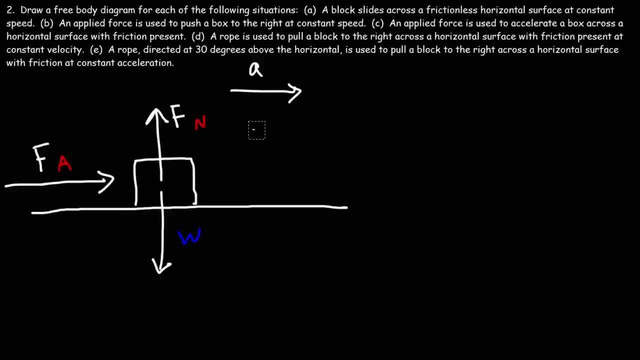 so kinetic friction has to be relatively small compared to the applied force so that we can have a net acceleration to the right. so this is going to be the free body diagram for part c. now what about part d? a rope is used to pull a block to the right across a horizontal surface. 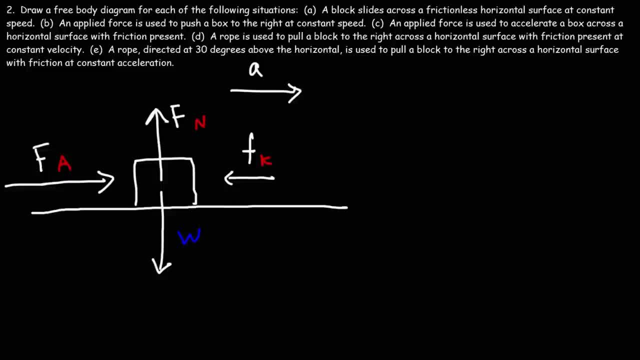 with friction present at constant velocity. so the normal force and the weight force will still be the same for part d. we no longer have an acceleration, we're moving at constant velocity, so the forces in the x direction must be balanced. this time we're using a rope. 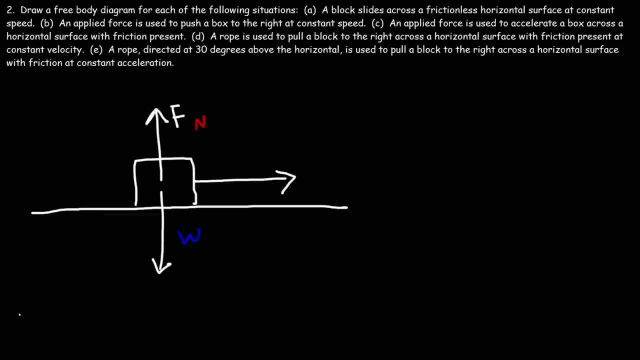 to pull the block to the right. so that's going to be our tension force and that's going to. the block is being pulled to the right against friction. friction always opposes motion. so if we're moving to the right, friction is going to be directed to the left. 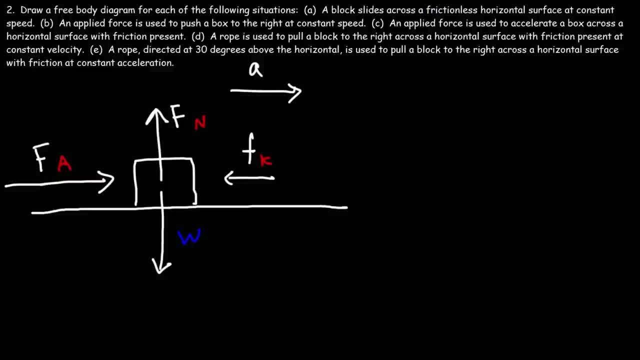 Now what about Part D? A rope is used to pull a block to the right across a horizontal surface with friction present at constant velocity. So the normal force and the weight force will still be the same For Part D. we no longer have an acceleration. 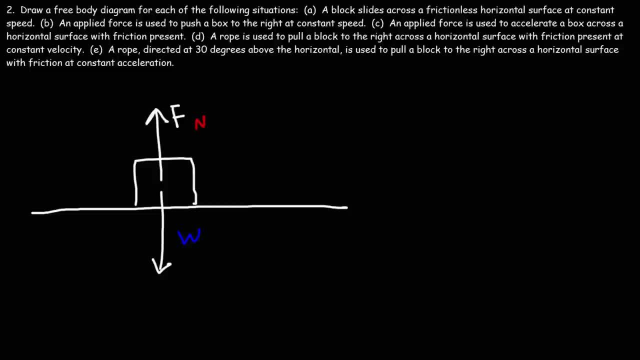 We're moving at constant velocity, so the forces in the x-direction must be balanced. This time we're using a rope to pull the block to the right, So that's going to be our tension force And that's going to. The block is being pulled to the right against friction. 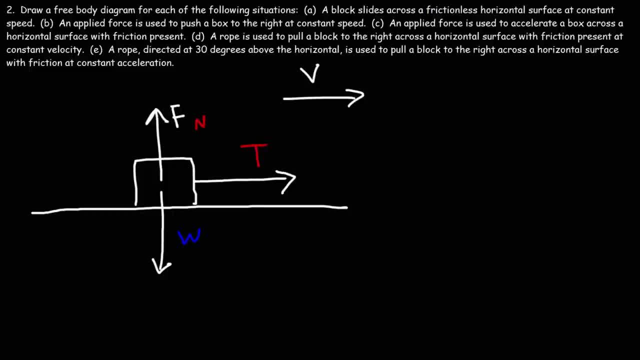 Friction always opposes motion, So if we're moving to the right, Friction is going to be directed to the left. So in this case, FK is going to be over here And it's going to have the same length as the tension force vector. 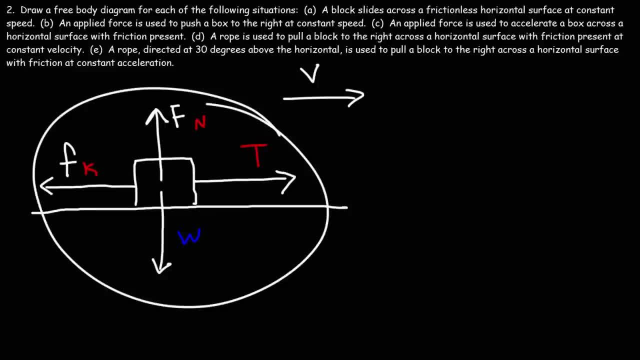 So this is the free body diagram that corresponds to the situation, the situation in Part D. Now let's move on to Part E. A rope directed at 30 degrees above the horizontal is used to pull a block to the right across a horizontal surface with friction present at constant velocity. 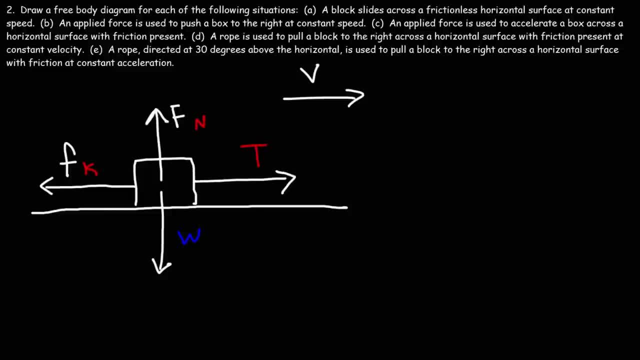 across a horizontal surface with friction at constant acceleration. So we no longer have constant velocity. We're going to accelerate the block to the right, So the forces in the X direction will not be equal. Now, if we're pulling the block to the right, 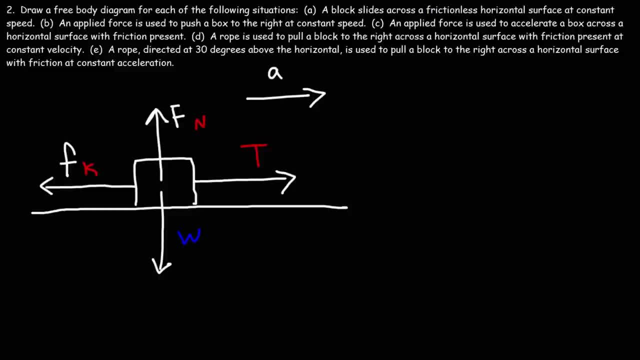 friction will still be directed towards the left, But if we're pulling it to the right with an acceleration, friction is going to be less than the tension force. So we're going to draw a relatively small FK value to left and a large tension force to the right, but at an angle. 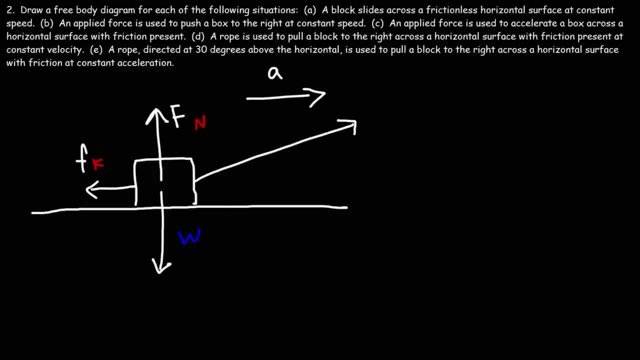 So we're going to draw a relatively small FK value to the left so that tension force has an X component and it has a Y component. It's directed at an angle of 30 degrees above the horizontal. The X component of the tension force is TX. 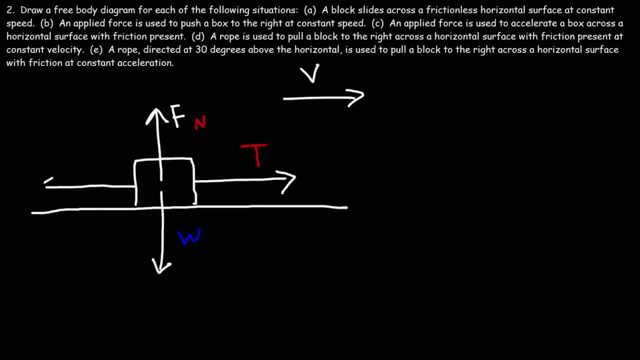 so in this case, fk is going to be over here and it's going to have the same length as the tension force vector. so this is the free body diagram that corresponds to the situation. the situation part d. now let's move on to part e. a rope directed at 30 degrees above the horizontal is used. 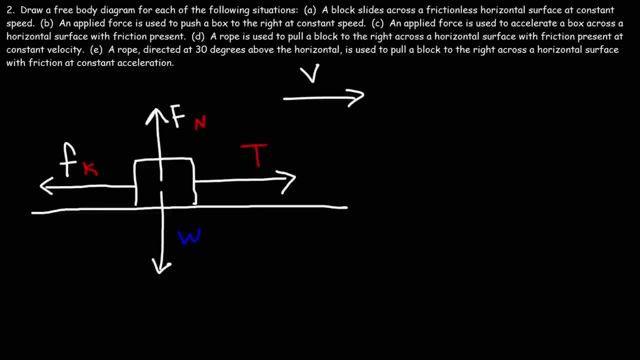 to pull a block to the right across a horizontal surface with friction at constant acceleration, so we no longer have constant velocity. we're going to accelerate the block to the right, so the forces in the x direction will not be equal. now, if we're pulling the block to the right, we're going to have a force that's going to 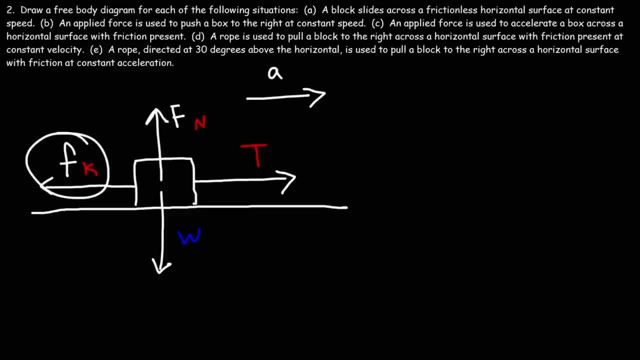 pull the block to the right, friction will still be directed towards the left. but if we're pulling it to the right with an acceleration, friction is going to be less than the tension force. so we're going to draw a relatively small fk value to the left and 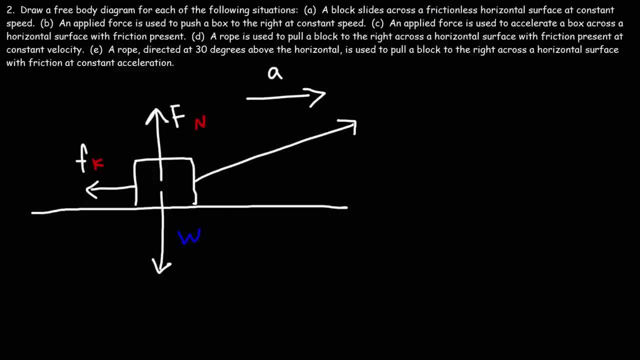 a large tension force to the right, but at an angle so that tension force has an x component and it has a y component. it's directed at an angle of 30 degrees above the horizontal. the x component of the tension force is tx and ty is the y component. 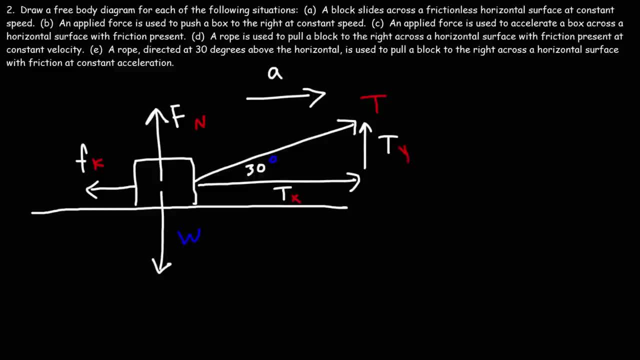 in order to accelerate the tension force, we're going to have to pull the block to the right. tx has to be greater than fk. now, in other problems the normal force was equal to mg, but that's not going to be the case in this example because of the y component of t. 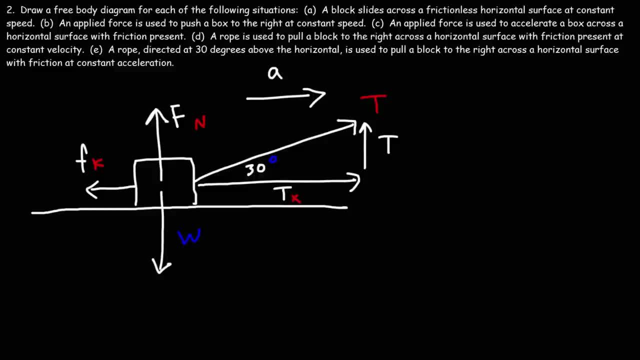 and TY is the Y component. In order to accelerate the block to the right, TX has to be greater than TX, TX has to be greater than TX And TX is going to be greater than FK And TX is going to be greater than FK. 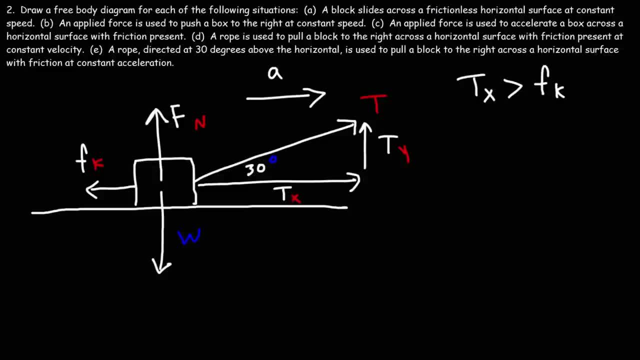 Now, in other problems the normal force was equal to MG, But that's not going to be the case in this example. because of the Y component of T, The block is not accelerating upward or downward, So the net force in the Y direction is zero. 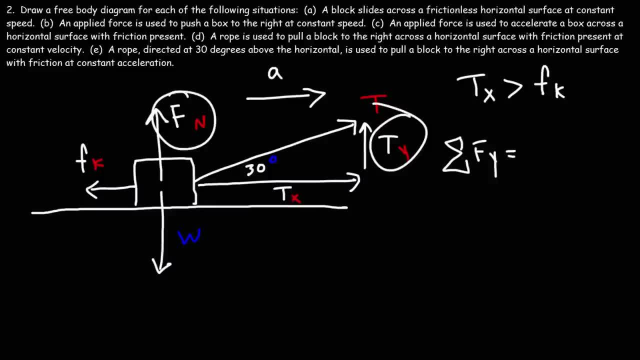 And it's equal to these two upward forces, which is positive Fn plus positive Ty, and then we have a downward force. so this is going to be negative W. now, because the block is not accelerating upward or downward, as was mentioned before, the net force in the y-direction is zero. 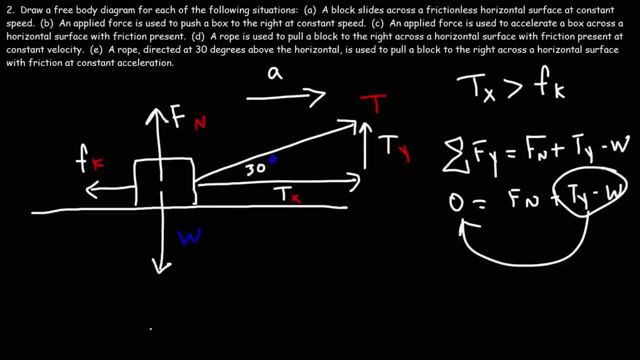 so if we take these two terms, move it to the other side, we'll get that the normal force is equal to Ty. it's actually going to be W positive W minus Ty. so the normal force is not mg in this problem. the normal force is the weight force, mg. but 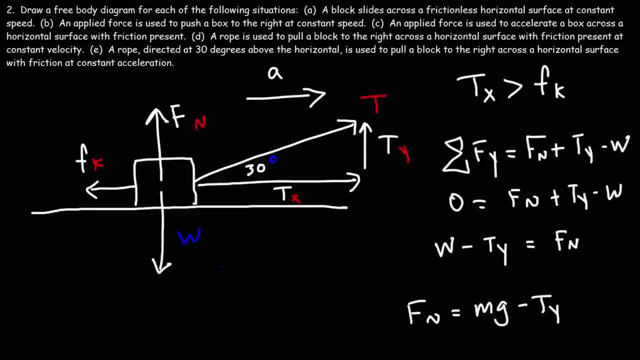 minus the y component of the tension force. so that's how you can calculate the normal force for this particular situation. now, what about calculating the acceleration of the block in the x-direction? how can we come up with a formula that's going to help us to get that answer? 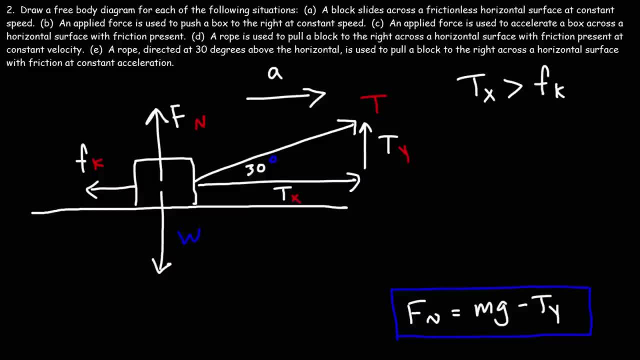 before we do that, let's talk about how to get Ty and Tx using SOHCAHTOA and trigonometry. Ty is equal to T sine theta, Tx is equal to T sin theta. Tx is equal to T cosine theta. so, going back to trig, we have the expression SOHCAHTOA. 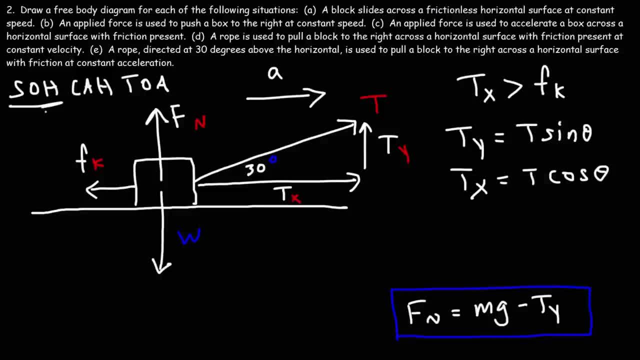 the SOH part means sine is equal to the opposite side over the hypotenuse. so sine of the angle theta- theta is 30 degrees in this example- is equal to opposite, which is Ty divided by the hypotenuse, which is T. the hypotenuse is: 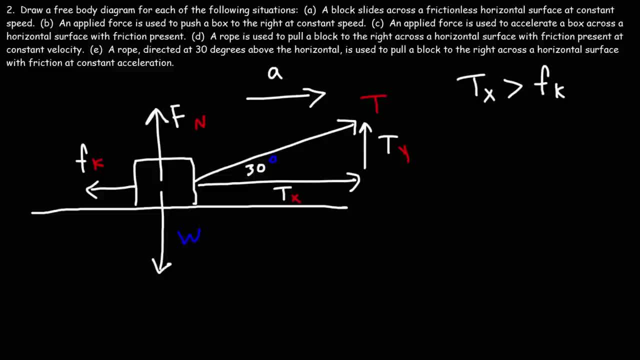 the block is not accelerating upward or downward, so the net force in the y direction is 0 and it's equal to t Și these two upward forces, which is positive Fn plus positive Ty, and then we have a downward force. so this is going to be negative W now because the block 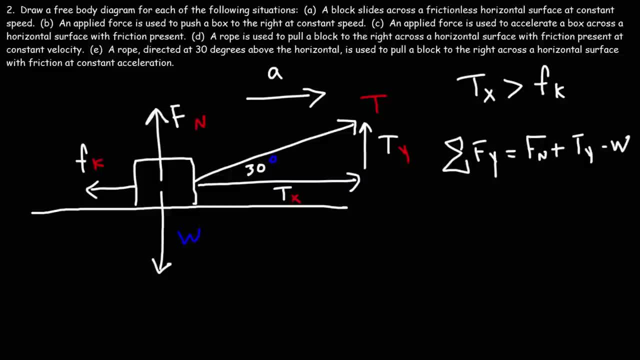 is not accelerating upward or downward. as was mentioned before, the net force in the y-direction is zero. so if we take these two terms, move it to the other side will get that the normal force is equal to ty is actually going to be W positive W minus ty. so the 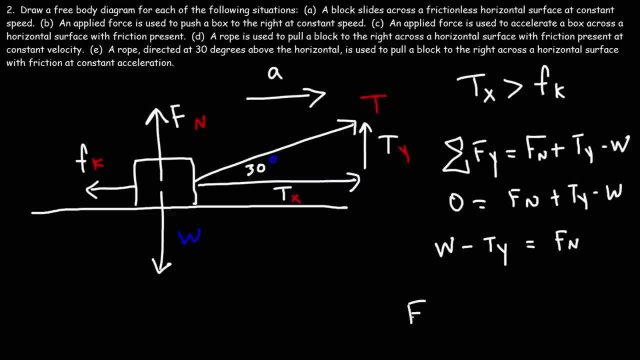 normal force is not mg. in this problem, the normal force is the weight force, mg, but minus the y component of the tension force. so that's how you can calculate the normal force for this particular situation. now, what about calculating the acceleration of the block in the x-direction? how can we come up with a formula that's going to? 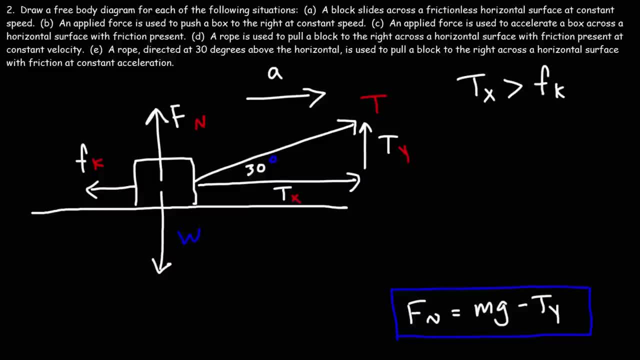 help us to get that answer. before we do that, let's talk about how to get ty and Tx using SOHCAHTOA and trigonometry. ty is equal to T sine theta, Tx is equal to T cosine theta. so, going back to trig, we have the expression SOHCAHTOA. the SOH part means 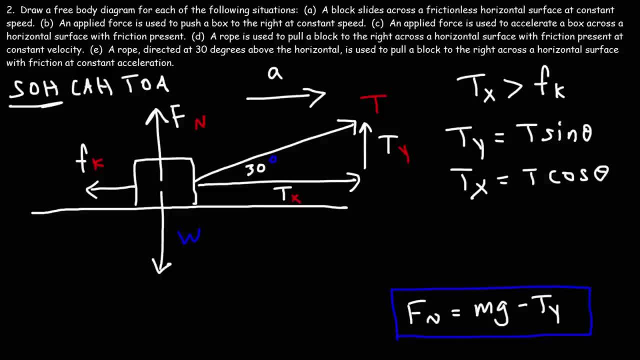 sine is equal to the opposite side over the hypotenuse. so sine of the angle theta- theta is 30 degrees in this example- is equal to opposite, which is ty divided by the hypotenuse, which is T. the hypotenuse is across the right angle, is the longest side of the triangle and so 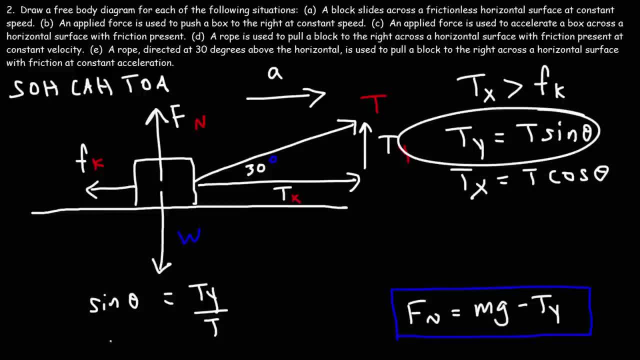 if you multiply both sides by T, you get: ty is equal to T sine theta. for the other equation we have cosine theta. so this is the club part. cosine is equal to the adjacent side divided by the hypotenuse, which is T. so multiplying both sides by T, you get. 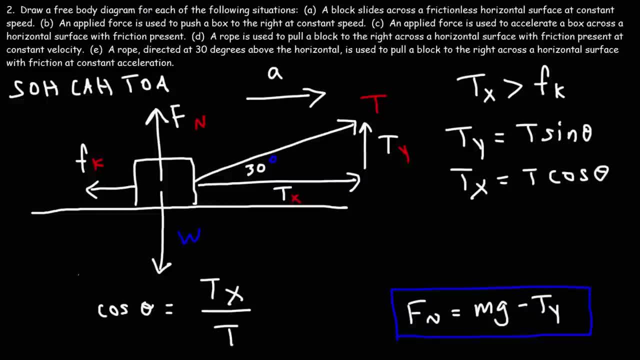 Tx is equal to T cosine theta. so that's how you can get Tx and Ty in this problem, if you know T, so you can plug T sine theta into this formula to get the normal force. but now to get the acceleration in the x-direction, we need to start with this expression. 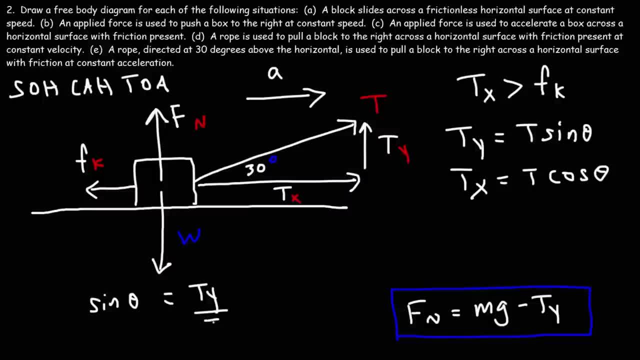 across the right angle. it's the longest side of the triangle and so if you multiply both sides by T, you get Ty is equal to T sin theta. for the other equation we have cosine theta. so this is the CAH part. cosine is equal to the adjacent side divided by the. 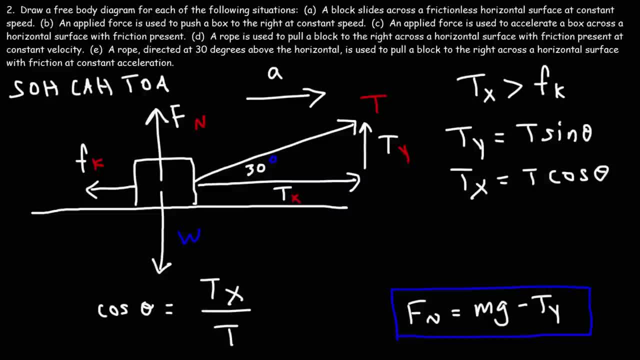 hypotenuse, which is T. so multiplying both sides by T you get T. X is equal to T cosine theta. so that's how you can get T X and T Y in this problem. if you know T, so you can plug T sine theta into this formula. to: 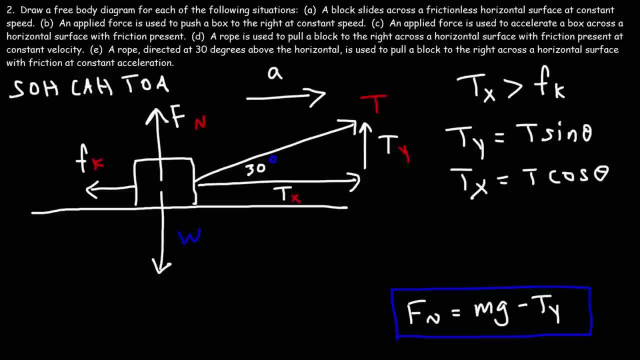 get the normal force. but now to get the acceleration in the X direction, we need to start with this expression: the sum of the forces in the X direction is T: X. it's positive because it's going to the right. this is negative because it's going to the left. so it's T? X minus F? K. now the net force, which is the sum of: 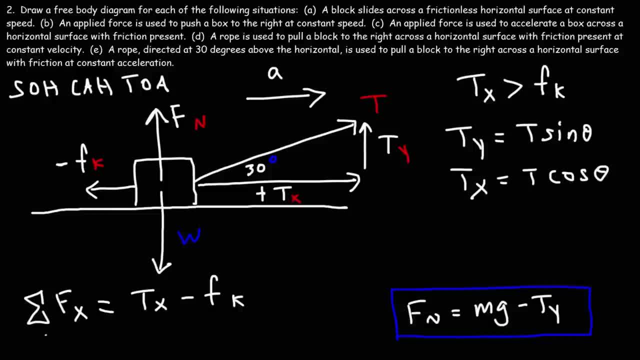 the forces is always equal to ma, based on Newton's second law. so this is going to be M, a sub X acceleration in the X direction. T. X is T cosine theta. now F, K is equal to mu K times the normal force, and this example might look a little bit complicated, but it's not. it's just an example of a. 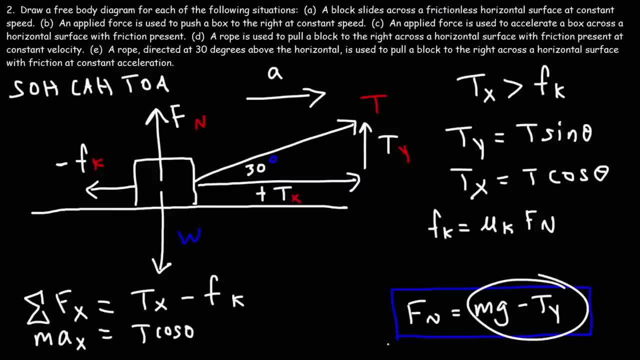 number. the normal force is not just mg, it's mg minus T Y. so I'm going to leave it like this. so first you want to calculate T X and T Y. once you have that, calculate the normal force. when you have the normal force, you have everything you. 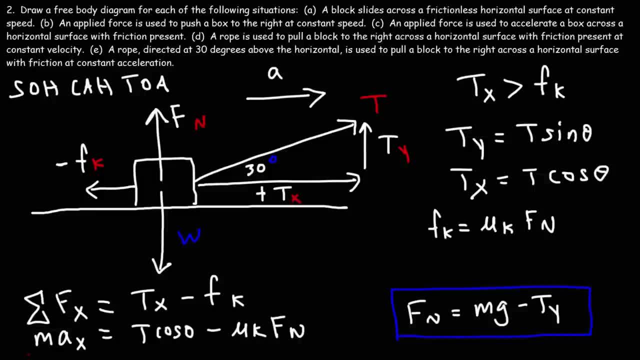 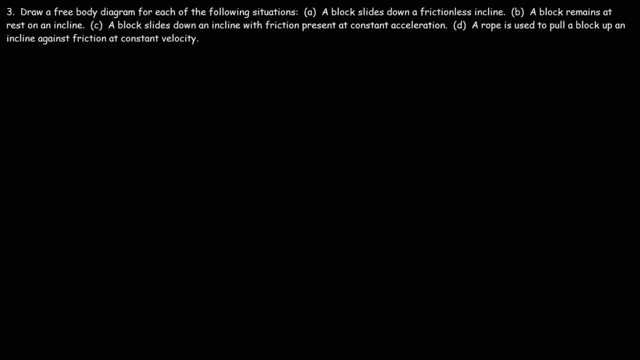 need to calculate the acceleration in that equation. so that's how we can find the acceleration in the X direction. it's by using that formula. now let's find the slope 0 and 0 and keep on working until we get to a point where it tells: 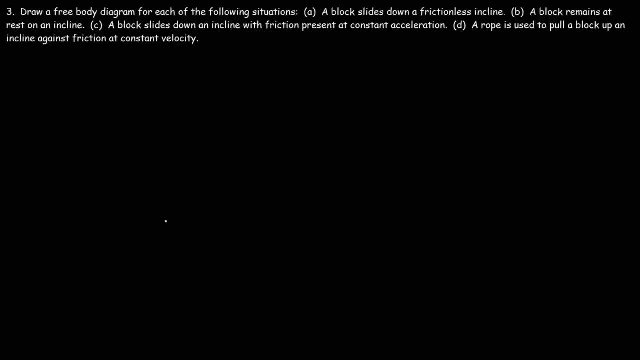 us that the x's get adjusts and it is approximately 1 square. once you get to, 1 square is exactly 1 square. so you are on the x's side. so the x's side is sinks, and so you- this is our x one- you have a perspectivists하시는. 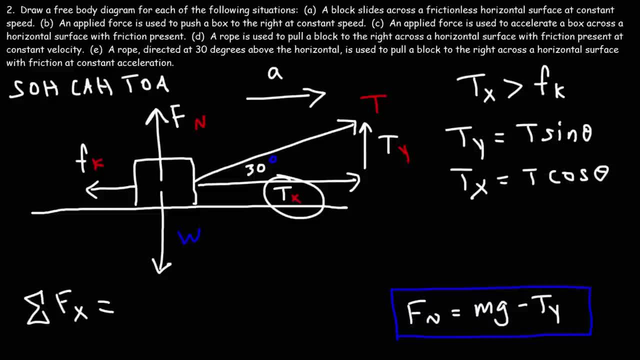 the sum of the forces in the x-direction is Tx. its positive because it is going to the right. This is negative because it's going to the left. So it's Tx minus Fk. Now the net force, which is the sum of the forces, is always equal to ma, based on Newton's second law. 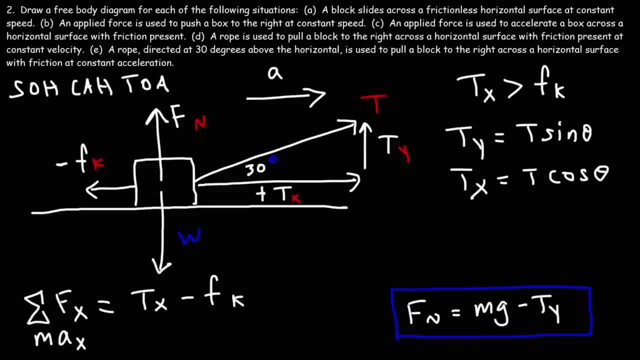 So this is going to be ma sub x acceleration in the x direction. Tx is T cosine theta. Now Fk is equal to mu k times the normal force. In this example, remember, the normal force is not just mg, it's mg minus Ty. 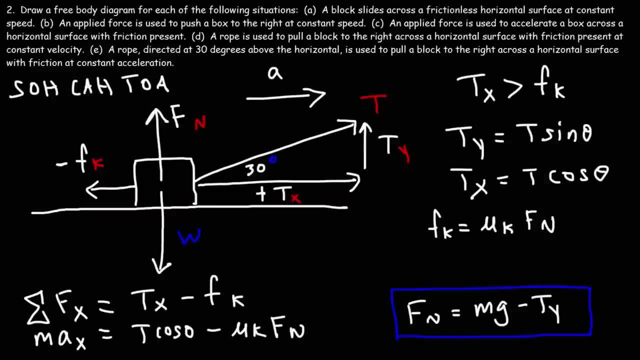 So I'm going to leave it like this. So first you want to calculate Tx and Ty. Once you have that, calculate the normal force. When you have the normal force, you have everything you need to calculate the acceleration in that equation. So that's how we can find the acceleration in the x direction. 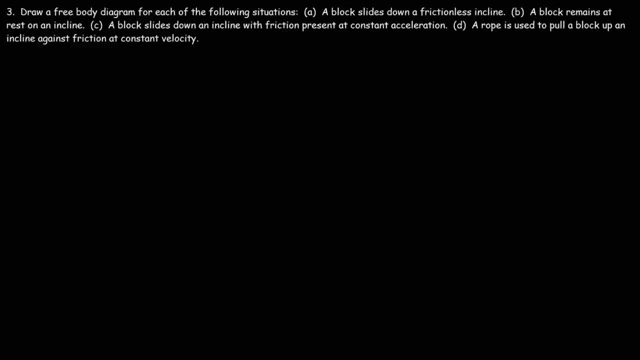 It's by using that formula. Now let's focus on free body diagrams with inclines. So part A: a block slides down a frictionless incline. Let's draw a picture. So here is our incline And here is the box on the incline. 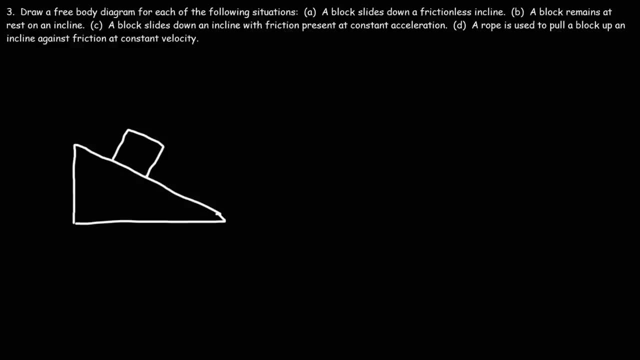 What forces are acting on this box? What forces are acting on this box? Let's see. So we have a downward weight force- We can just call that W- And we have a normal force. The normal force is less than the weight force. 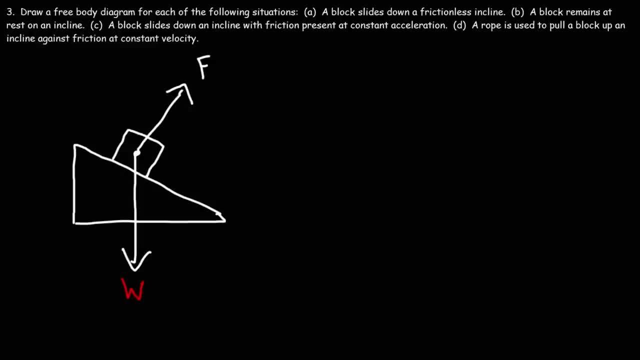 So that arrow should be smaller than W, W, W, W. The extension extent to which, like how much smaller, depends on the angle of the incline. as the angle of the incline increases, Fn becomes much smaller relative to W. so on an incline the normal force is going to be mg, cosine theta as the angle. 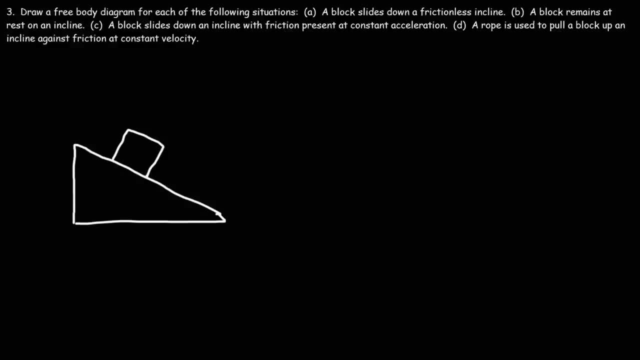 so we're explaining what flats just means: 100 masses and the ole just is. this is all the math I gave you so far and we have pretty much covered all of it. we have created all of about 32 levels which can look okay, but before we 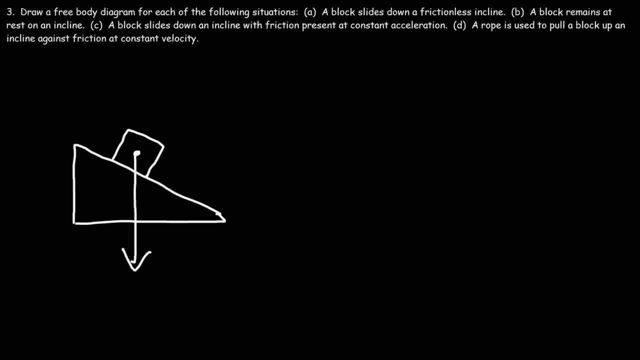 dive deeper into it. I want to say something helpful here to help you understand properly. what is it all about. this is page 4. image 1 will be in the sub and certainly at day 2. it's when we talk about putting the negative force. we can just call that W and we have a normal force. the normal force is: 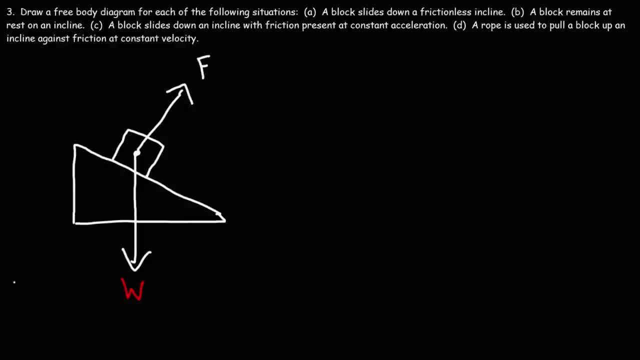 less than the weight force, so that arrow should be smaller than W. the extent to which like how much smaller depends on the angle of the incline. as the angle of the incline increases, Fn becomes much smaller relative to w. so on an incline the normal force is going to be mg cosine theta as the angle increases from. 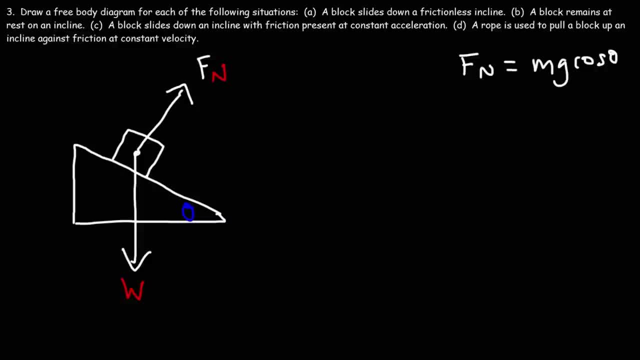 0 to 90. cosine decreases from 1 to 0. so as theta goes up, from zero to 90, the normal force goes down. so the left of this arrow will get smaller as theta increases. now what other forces do we have acting on this picture, or the? 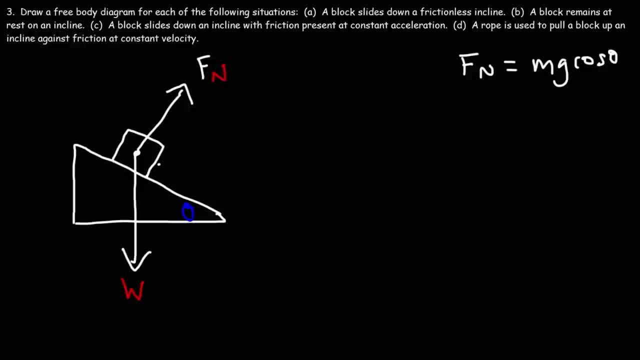 block. now we have a component of gravity that will accelerate the block down the incline, and I'm going to call that FG. FG is equal to mg sine theta, so as the block slides down on an incline that does not have friction, it's not going. 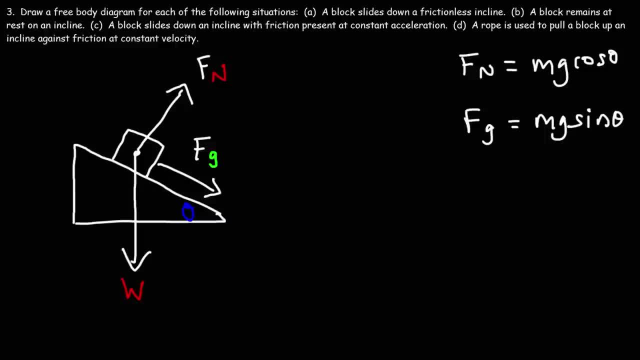 down at constant speed. it's accelerating downward. the only way you can go down at constant speed is if friction is present and if it's equal to FG. but because friction is not present, this is the only force acting parallel to the incline, so there is an acceleration to calculate. 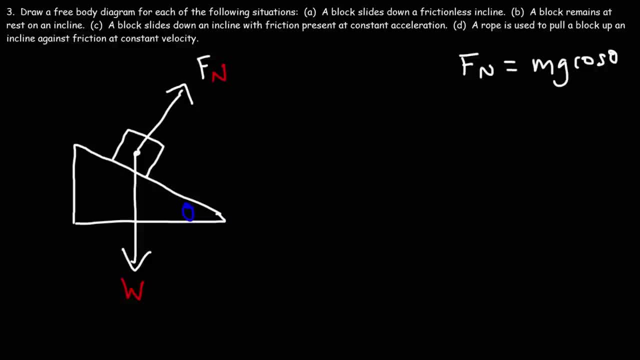 increases from 0 to 90. cosine decreases from 1 to 0. so as theta goes up from 0 to 90, the normal force goes down. so the left of this arrow will get smaller as theta increases. now what other forces do we have acting on this picture or the block? now we have 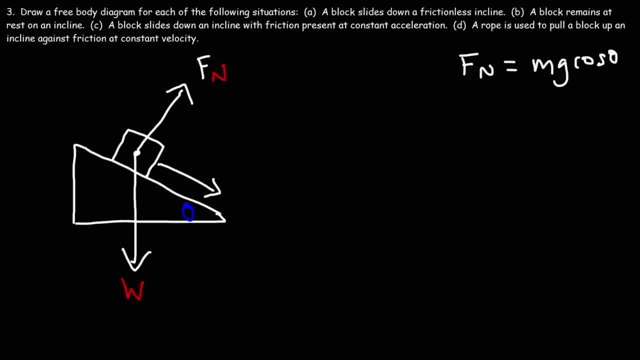 a component of the normal force that we have acting on this picture, or the block gravity that will accelerate the block down the incline, and I'm gonna call that Fg. Fg is equal to mg sine theta, so as the block slides down on an incline, that 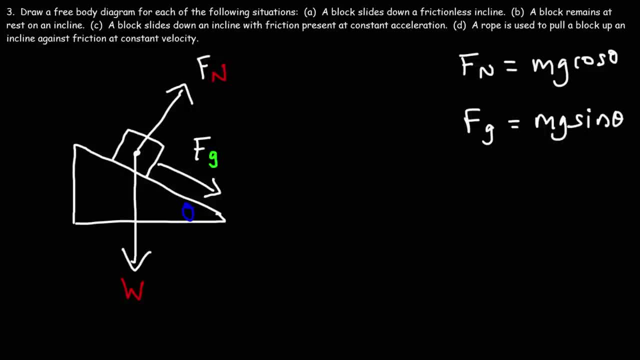 does not have friction, it's not going down at constant speed, it's accelerating downward. the only way you can go down at constant speed is if friction is present and if it's equal to Fg. but because friction is not present, this is the only force acting parallel to the incline, so there is an acceleration. to calculate that: 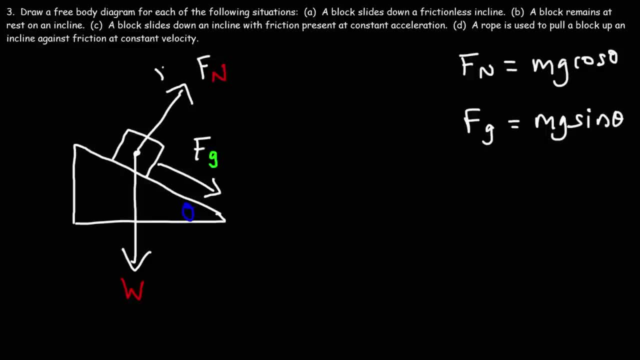 acceleration. let's define this as the y-axis, and this has the x-axis with respect to the block. so the sum of the forces in the x-direction is equal to Fg. that is the only force acting along the x-axis, parallel to the incline, and this is always equal to ma. 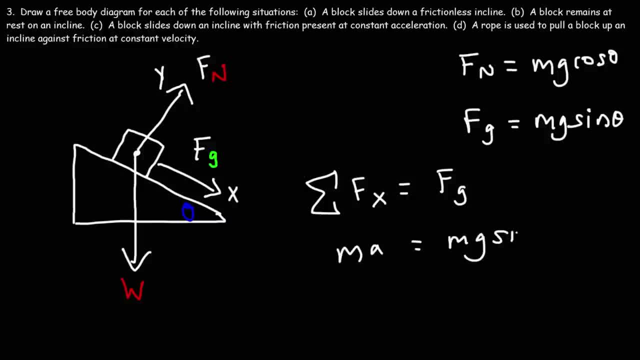 Fg is Mg sine theta, so we could divide both sides by M, so those variables will cancel, thus the acceleration. for this problem, part a is simply equal to G sine theta. so that's how you can calculate the acceleration of a block that slide and down a frictionless incline. Now for those of you who might be wondering how we can get these: 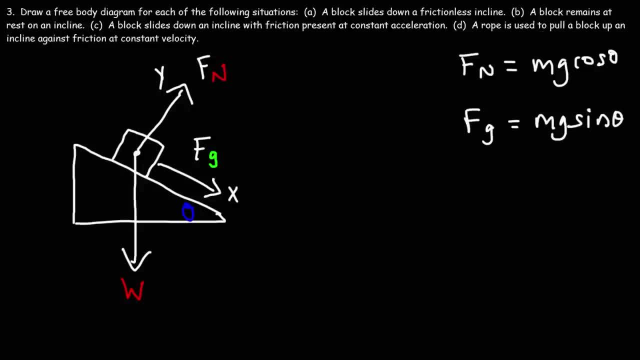 equations. here's what you can do. So draw a line that is parallel to the normal force. We're going to create a triangle where W is the hypotenuse of that triangle. So let me just put this in a different color so you can see it. 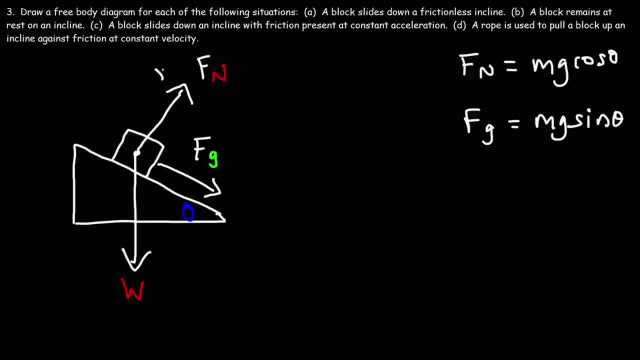 that acceleration. let's define this as the y-axis and this has the x-axis with respect to the block. so the sum of the forces in the x-direction is equal to FG. that is the only force acting along the x-axis, parallel to the incline, and this is always equal to ma. FG is mg sine. 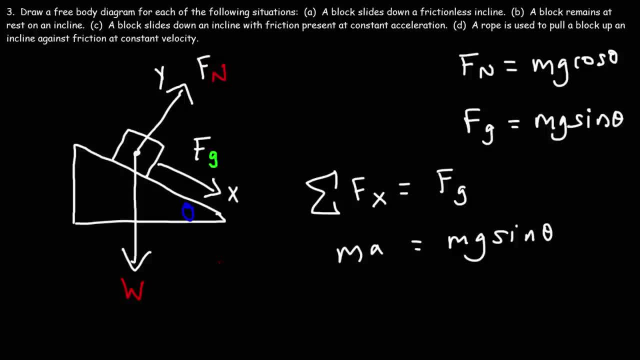 theta, so we could divide both sides by M, so those variables will cancel thus the acceleration. for this problem, part a is simply equal to G sine theta. so that's how you can calculate the acceleration of a block that's sliding down a frictionless incline. now for those of you who might be wondering how we can get these equations: 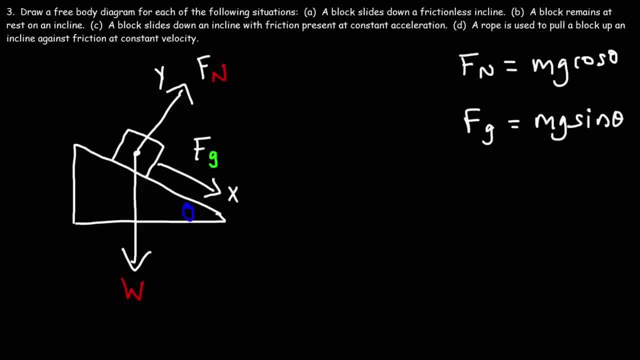 here's what we can do. so draw a line that is parallel to the normal force. we're going to create a triangle where W is the hypotenuse of that triangle. so let me just put this in a different color so you can see it, you, you? 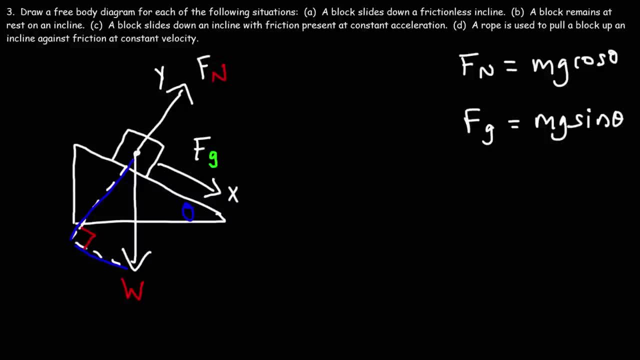 So there's the triangle and here's the right angle And this angle, theta is equivalent to this angle. So across theta, that's the opposite side. We know that sine is opposite over hypotenuse, So I'm going to redraw this triangle. 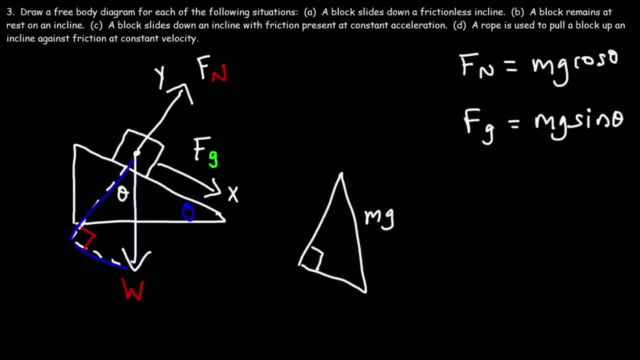 So the hypotenuse is the weight force, which is mg. This is theta Across theta. this is going to be mg sine theta, And on the adjacent side, cosine is associated with the adjacent side. So this side here, that's going to be mg, cosine, theta. 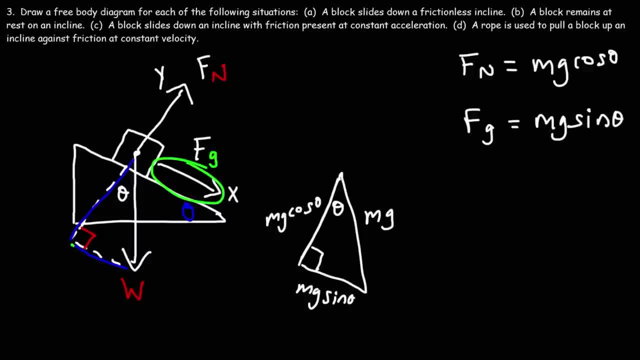 So notice that Fg is equal to this component of gravity Because that component is parallel to Fg. So that's why Fg is equal to this component of gravity. Fg is equal to mg sine theta. The normal force balances this portion of the triangle. 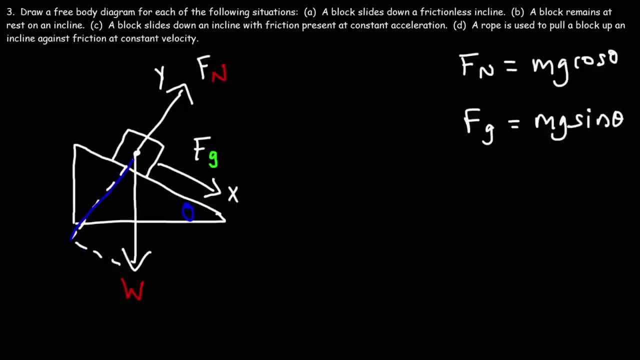 So there's the triangle and here's the right angle And this angle, theta is equivalent to this angle. So across theta, that's the opposite side. we know that sine is opposite over hypotenuse, So I'm going to redraw this triangle. So the hypotenuse is the weight force, which is mg. 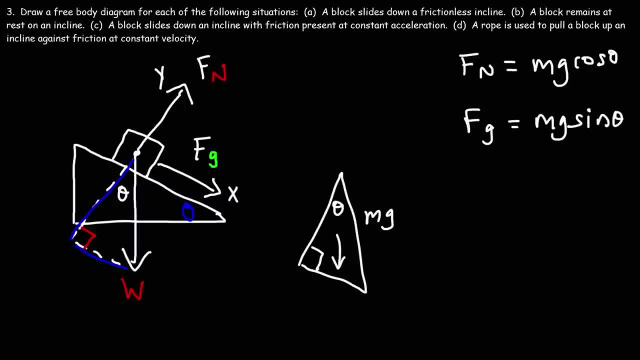 This is theta Across theta. this is going to be mg sine theta And on the adjacent side, cosine is associated with the adjacent side. So this side here, that's going to be mg cosine theta. So notice that Fg is equal to this component of gravity because that component is parallel to Fg. 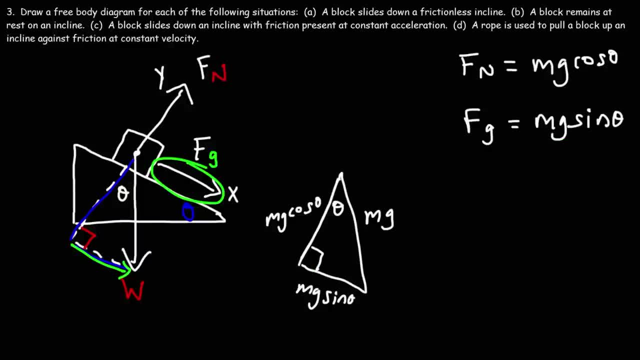 So that's why Fg is equal to mg sine theta. The normal force balances this portion of the triangle, So that's why the normal force is mg cosine theta. So that's how you can get those equations from that free body diagram. Now part B: 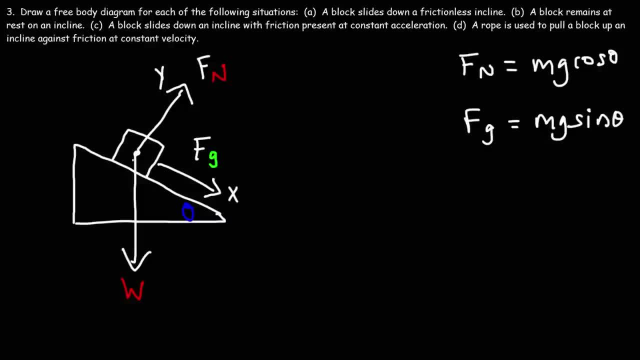 A block remains at rest. So the block is still on the incline. We're still going to have the normal force, the weight force and Fg. Those forces will always be present for an object on an incline. But this time, in part B, the block is not sliding down the frictionless incline. 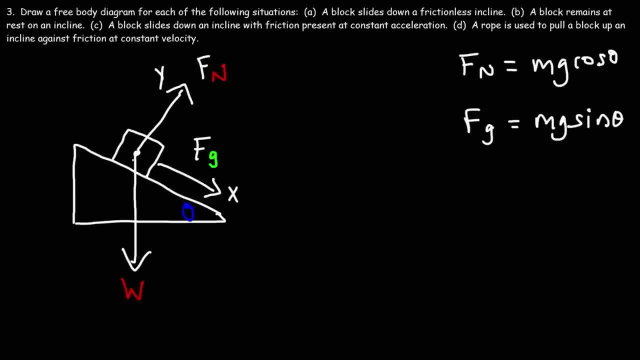 It's remaining at rest. The only way it can remain at rest is if the net force in the x direction is zero, So there must be some other force That's preventing it from sliding down, And that force must be equal in magnitude to Fg. 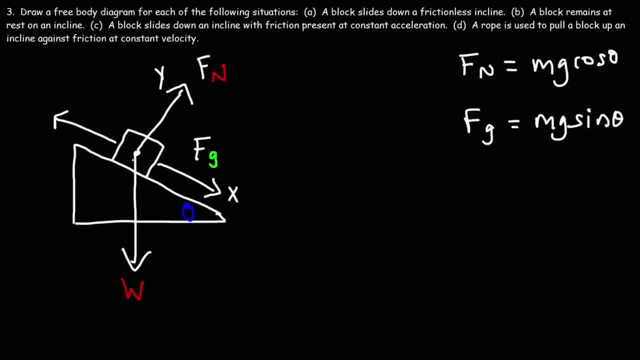 So what is that force? Well, that can only be friction. Friction opposes motion. Remember there's two types of frictional forces whenever you have objects like sliding past each other. You have kinetic friction when they're sliding past each other and static friction when they're at rest. 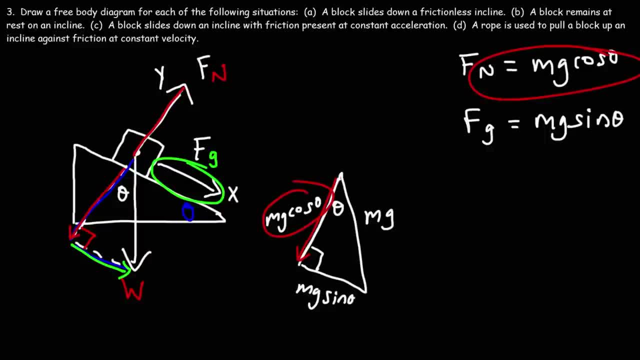 So that's why the normal force is mg, cosine theta. So that's how you can get those equations from that free body diagram. Now part B: A block remains at rest on an incline. So the block is still on the incline. 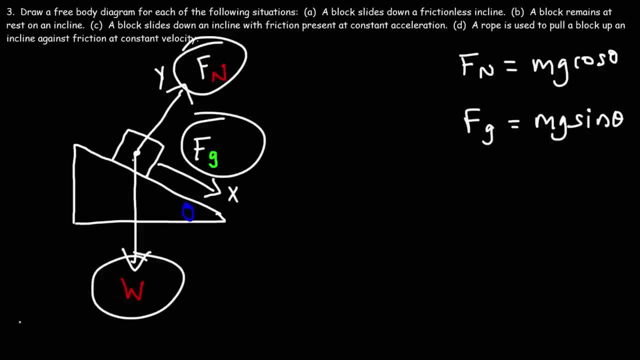 We're still going to have the normal force, the weight force and Fg. Those forces will always be present for an object on an incline, But this time, in part B, the block is not sliding down the frictionless incline. 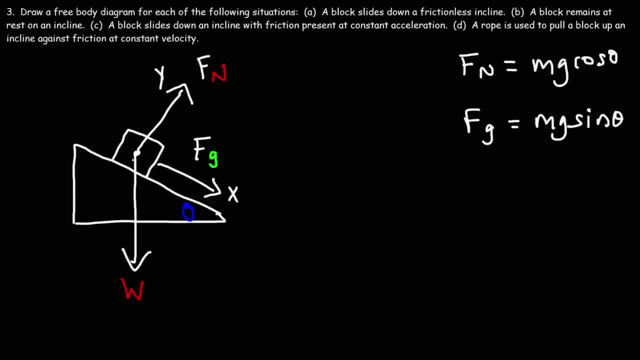 It's remaining at rest. The only way it can remain at rest is if the net force in the x direction is zero, So there must be some other force That's preventing it from sliding down, And that force must be equal in magnitude to Fg. 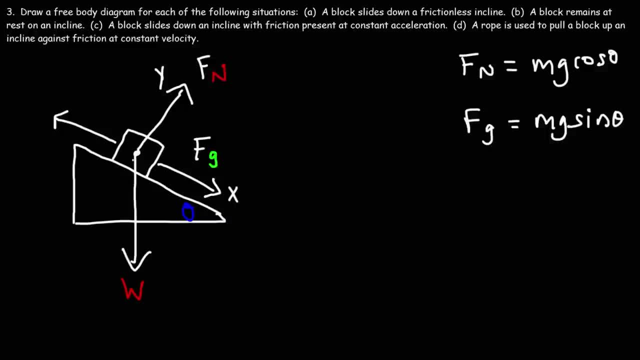 So what is that force? Well, that can only be friction. Friction opposes motion. Remember, there's two types of frictional forces. Whenever you have objects like sliding past each other, You have kinetic friction. when they're sliding past each other. 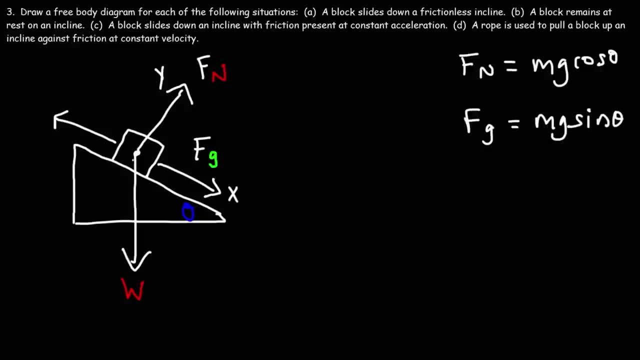 And static friction when they're at rest. So because the block is at rest, Static friction is the force that is going against Fg, That's preventing it from sliding down. So in this example Fs is equal to Fg. Now the static frictional force is less than or equal to μs times the normal force. 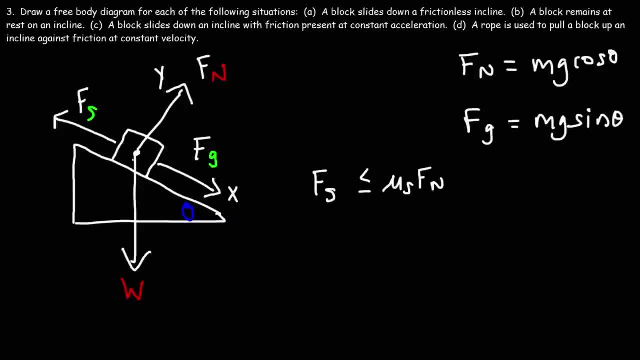 So static friction is an inequality. It's going to match Fg up to a maximum. So let's say that maximum is 100.. If we were to make a table that shows the relationship between Fg and Fs, If Fg is zero, Fs is zero. 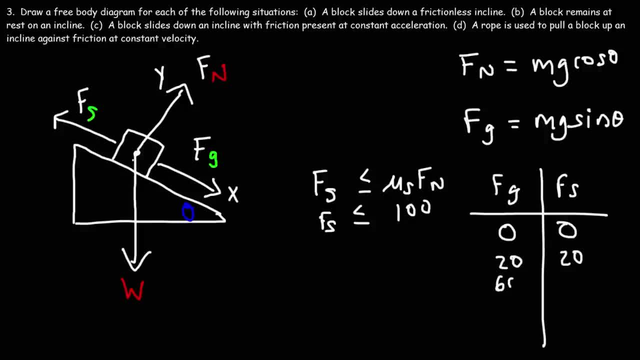 If Fg is 20, Fs is 20.. If Fg is 60, Fs is going to match it to 60.. If Fg is 100, Fs will be 100.. If Fg is 110, static friction has been exceeded. 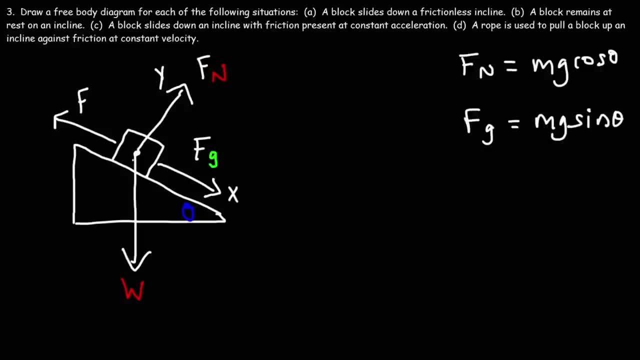 So, because the block is at rest, Static friction is the force that is going against Fg, that's preventing it from sliding down. So in this example, Fs is equal to Fg. Now the static frictional force is less than or equal to μs times the normal force. 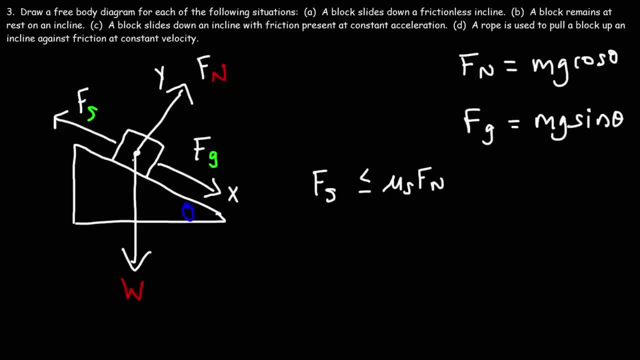 So static friction is an inequality. It's going to match Fg up to a maximum. So let's say that maximum is 100.. If we were to make a table that shows the relationship between Fg and Fs, if Fg is zero, Fs is zero. 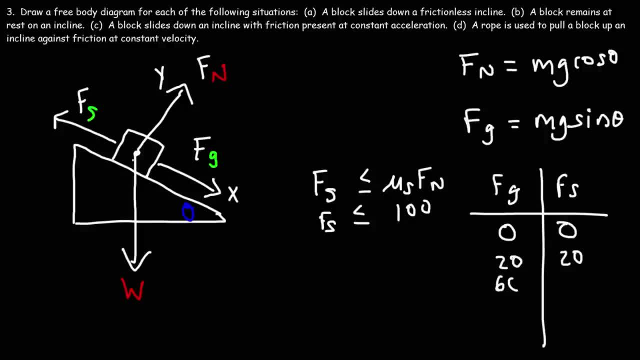 If Fg is 20, Fs is 20.. If Fg is 60, Fs is going to match it to 60.. If Fg is 100, Fs will be 100.. If Fg is 110, static friction has been exceeded. 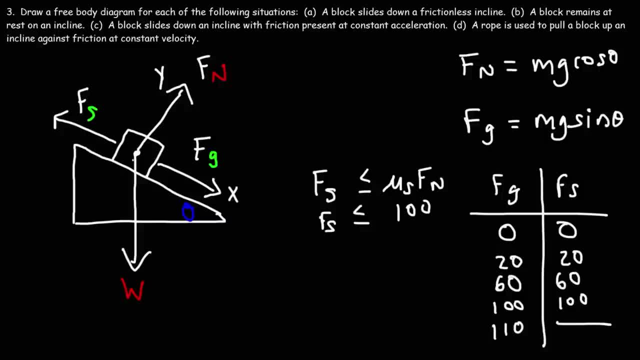 The block will begin to slide down and you're not going to have static friction anymore, You're going to have kinetic friction. So static friction will match Fg up to a certain limit, at which point the block will begin to slide down. But this is the free body diagram for part B. 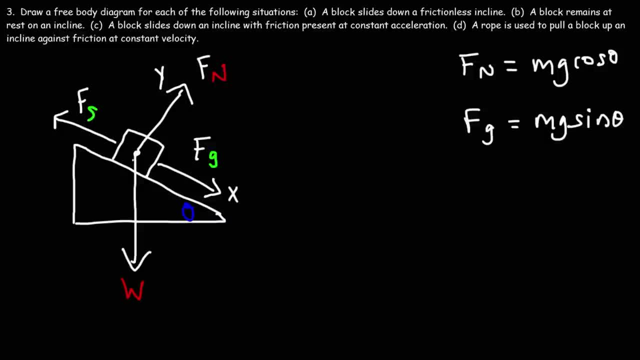 Now part C. A block slides down an incline with friction present at constant acceleration. So let's delete this. So there's constant acceleration, Which means Fg has to be greater than friction, And because the block is sliding down, we no longer have static friction, but we have 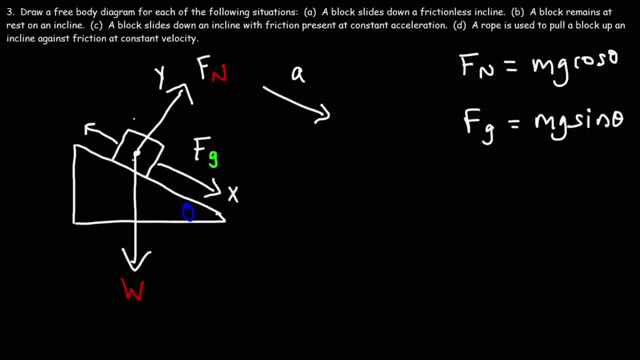 kinetic friction. so FK is going to be smaller than FG. now how can we calculate this acceleration? well, we can write this equation: the sum of the forces in the X direction is going to be FG minus FK. the net force in the X direction will always equal. ma we know FG is mg sine theta. FK, that's mu K times the normal. 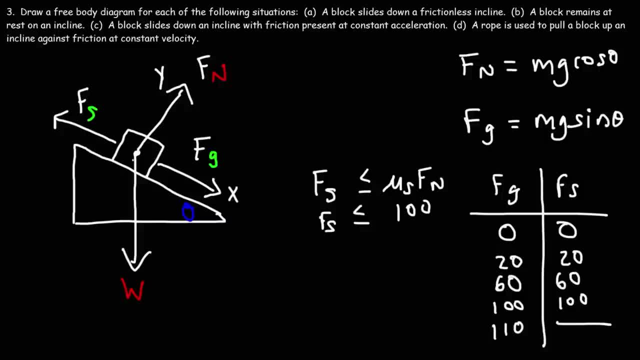 The block will begin to slide down and you're not going to have static friction anymore, You're going to have kinetic friction. So static friction will match Fg up to a certain limit, at which point the block will begin to slide down. But this is the free body diagram for Part B. 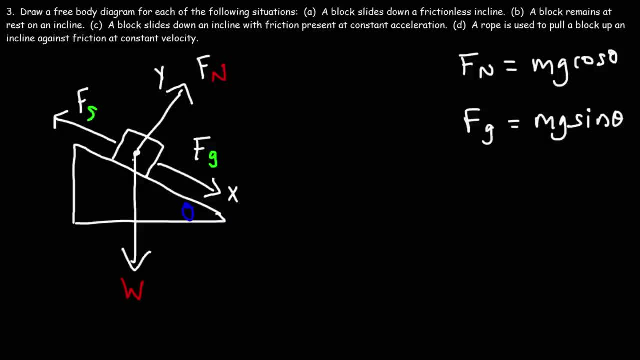 Now Part C. A block slides down an incline with friction present at constant acceleration. So let's delete this. So there's constant acceleration, Which means Fg has to be greater than friction. And because Fg is greater than friction, Fg has to be greater than friction. 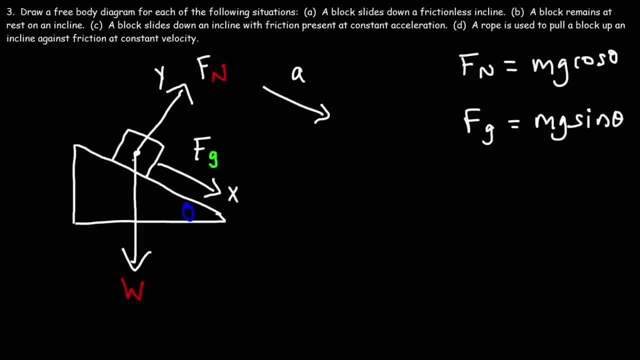 And because the block is sliding down, we no longer have static friction, but we have kinetic friction. So Fk is going to be smaller than Fg. Now how can we calculate this acceleration? Well, we can write this equation. 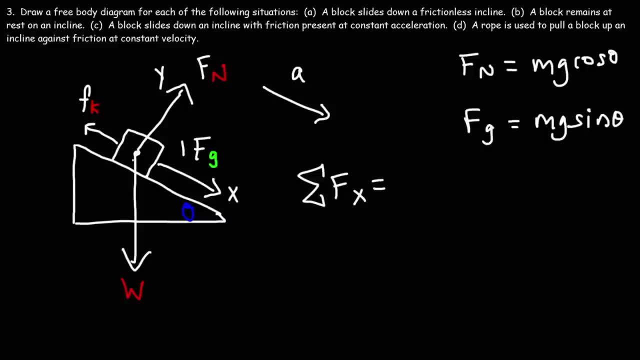 The sum of the forces in the x direction is going to be Fg minus Fk. Well, we can write this equation: The sum of the forces in the x direction is going to be Fg minus Fk. Well, we can write this equation: The sum of the forces in the x direction is going to be Fg minus Fk. 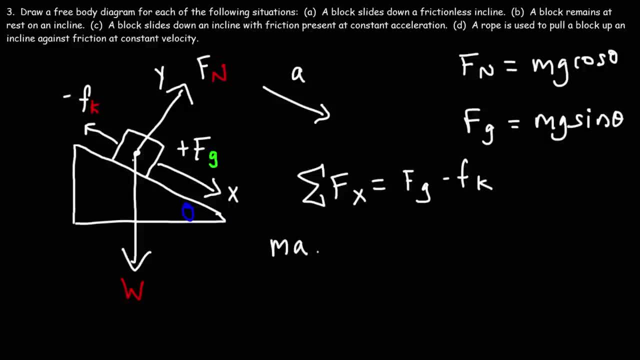 Well, we can write this equation: The sum of the forces in the x direction is going to be Fg minus Fk. The net force in the x direction will always equal. Ma We know Fg is Mg sine theta. Fk, that's mu k times the normal force. 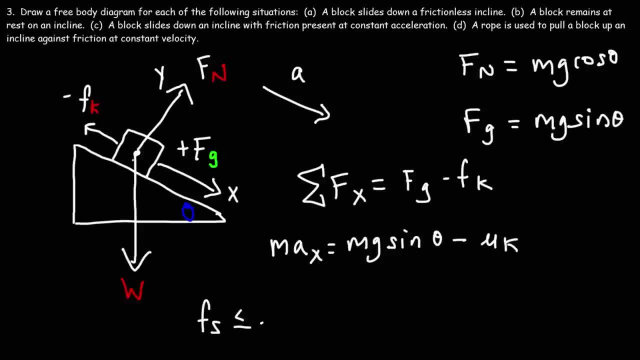 By the way, static friction Fs is mu s times the normal force, But notice that it's an inequality. It's going to match up. It's going to match Fg up to a certain limit. Fk does not have that inequality. 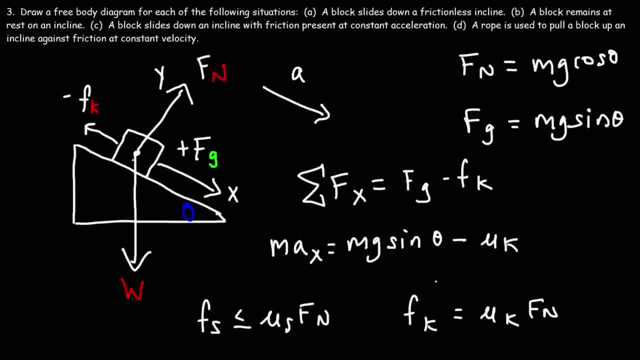 It's simply equal to mu k times the normal force. So this is a fixed value. It doesn't depend on the value of Fg. So make sure you're aware of that difference between Fs and Fk. So Fk is going to be mu k times the normal force. 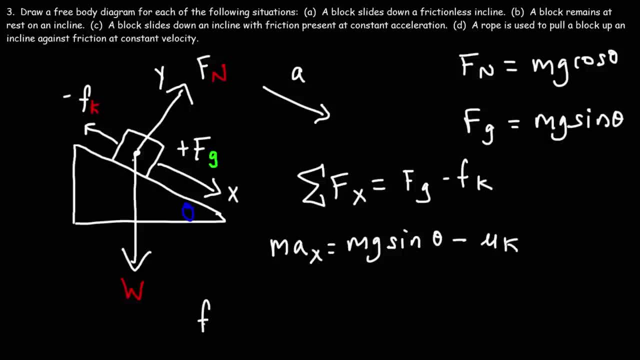 force. by the way, static friction FS is mu s times the normal force. you but notice that it's an inequality. it's going to match up. it's going to match FG up to a certain limit. FK does not have that inequality, it's simply equal to mu. 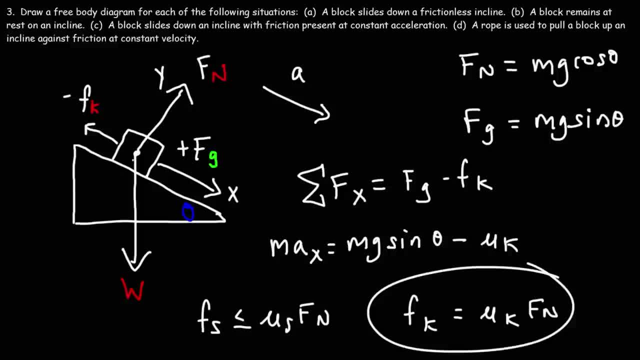 K times the normal force. so this is a fixed value. it doesn't depend on the value of FG. so make sure you're aware of that difference in between FS and FK. so FK is going to be mu K times the normal force and the normal force is mg cosine theta. so we can just 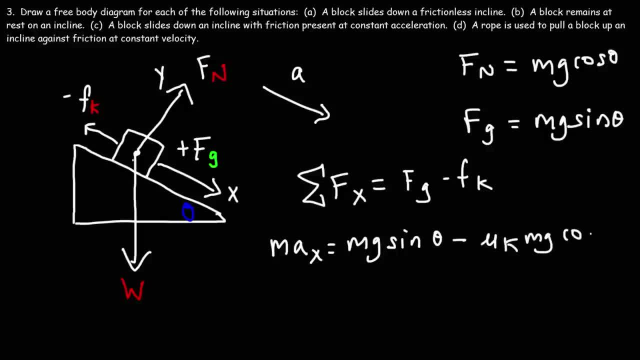 replace FN with mg cosine theta. since each term contains M, we can divide every term by M. therefore the acceleration in the X direction for this example is going to be G sine theta minus mu k g cosine theta. so that's how you can calculate it for this problem, that is, for Part C. now 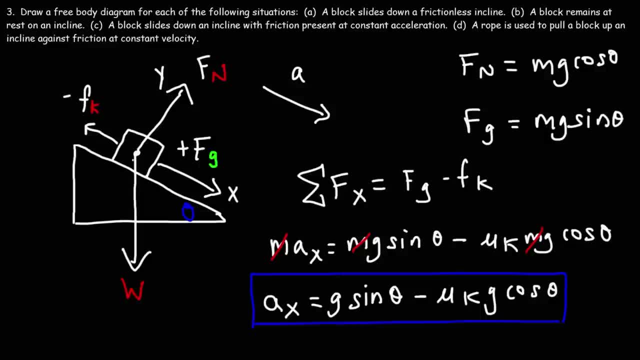 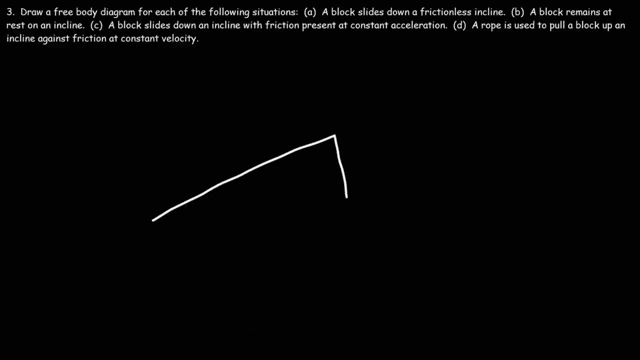 let's move on to Part D. a rope is used to pull a block up an incline against friction at constant velocity. feel free to try that problem. so let's draw a different incline. this time we're going to draw an incline that goes up as the 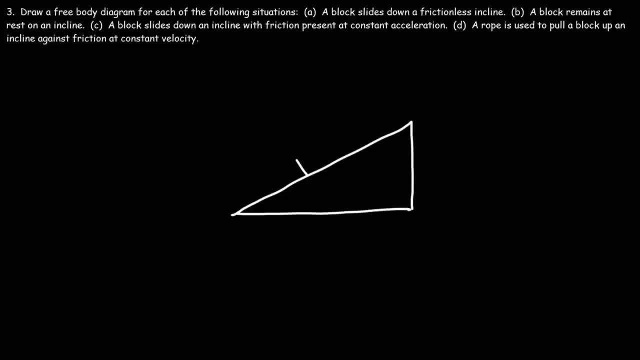 block moves to the right. so let's put the block here and we're gonna pull the block up an incline. so this is going to be our tension force. we still have our downward weight force and we're still going to have the normal force, which is going to be less than the. 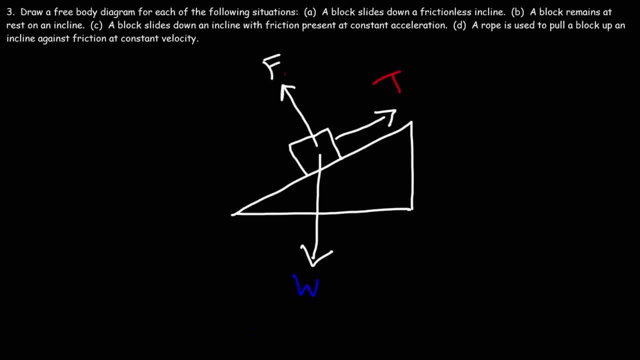 weight force as long as there's an angle, the only way they'll be equal if the angle is zero. so the angle is not zero for an incline. thus the normal force has to be less than the weight force. now we're pulling it up against friction at. 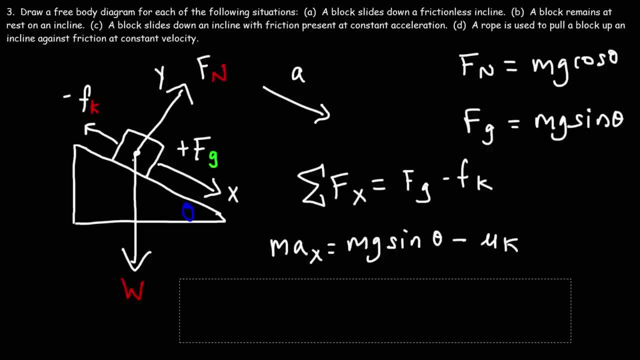 And the normal force is Mg cosine theta. So we can just replace Fg Fn with Mg cosine theta. Since each term contains M, we can divide every term by M. Therefore the acceleration in the x direction for this example is going to be g sine theta minus mu k: g cosine theta. 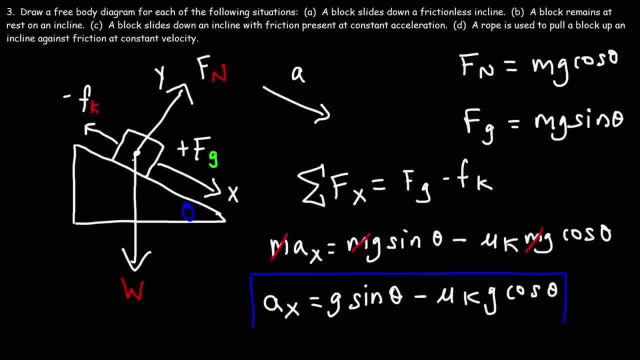 So that's how you can calculate it for this problem. That is for part C. Now let's move on to part D. A rope is used to pull a block up an incline against friction at constant velocity. Feel free to try that problem. 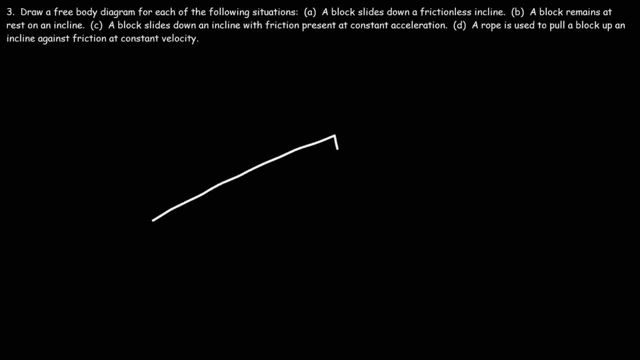 So let's draw a different incline. This time we're going to draw an incline that goes up as the block moves to the right. So let's put the block here And we're going to pull the block up an incline. 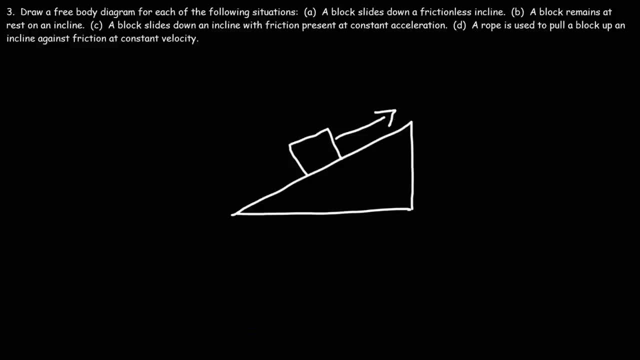 So this is going to be our tension force. We still have our downward weight force And we're still going to have the normal force, which is going to be less than the weight force, as long as there's an angle, The only way they'll be equal if the angle is zero. 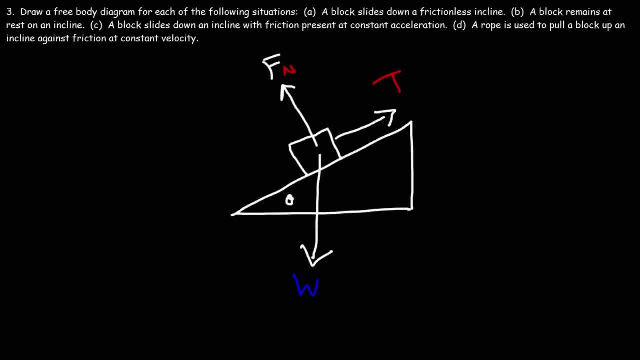 So the angle is not zero for an incline. Thus the normal force has to be less than the weight force. Now we're pulling it up against friction at constant velocity. So because it's moving, we're dealing with kinetic friction. 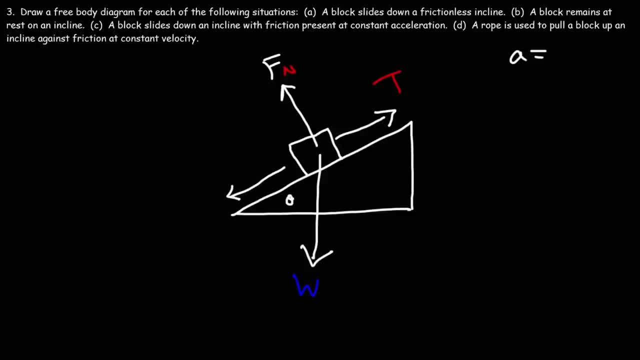 And because the velocity is constant, there's no acceleration. So the forces are balanced in the x direction, which means that tension force is equal to Fk. So if we wish to calculate the tension force in this case, we could say: the sum of the forces in the x direction is equal to positive T minus Fk. 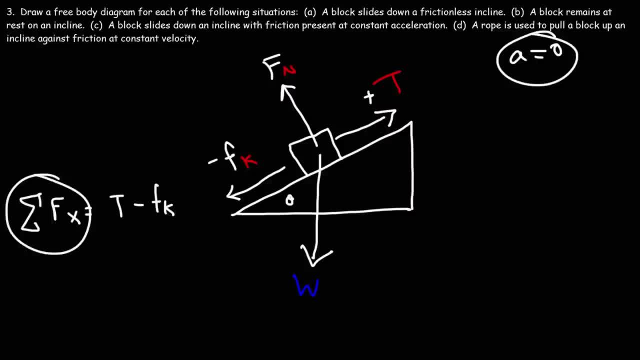 Now, because the acceleration is zero and this equals ma m times. zero is zero, So this is zero. Add an Fk to both sides. we get that Fk is equal to T, Or T is equal to T minus Fk.